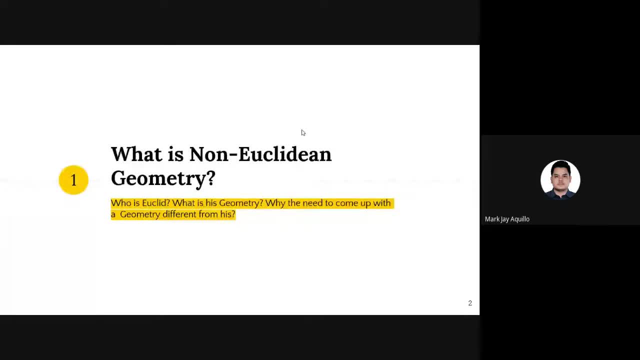 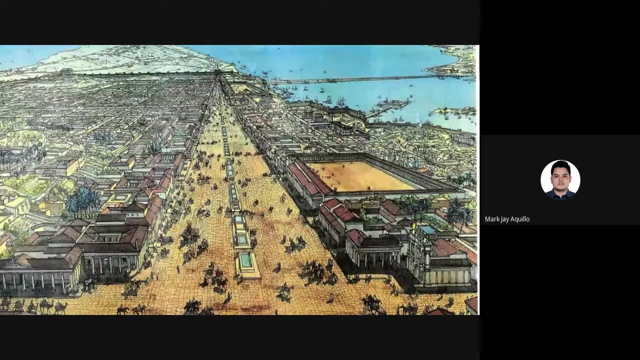 And why do we need to come up with a different geometry than the geometry of Euclid? Why the need for modern geometry? Is classical geometry not enough? Is modern geometry more fit To our times? we're going to find out One moment. try to fix the microphone. 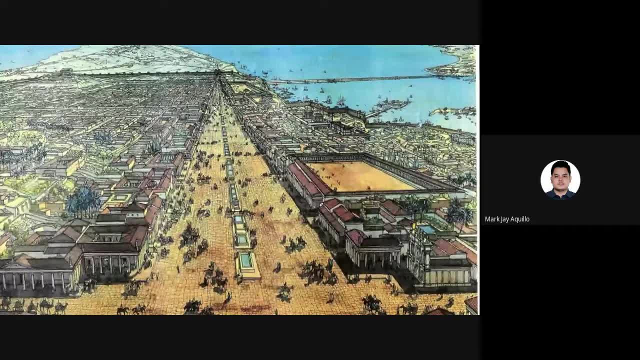 Hello, I'm sorry. I think there's a static in the aircon here. Now let's go back to the lesson. I'm showing you a famed city of Alexandria. Alexandria is one of the three big cities of Egypt. One is Cairo, Another is this Alexandria. The third one is Giza. Is it Giza, sir? Yeah, it's Giza. 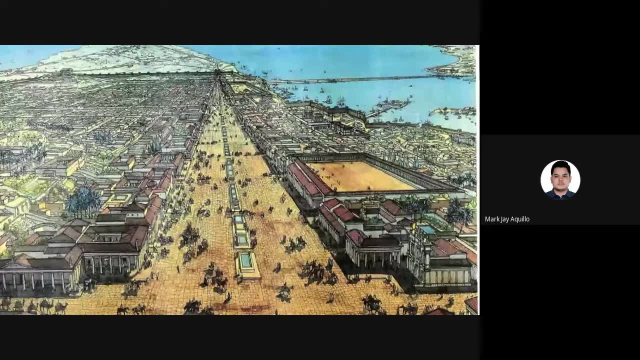 Famous for its pyramid. This one is also a famed city, a very big city in Egypt. We call it Alexandria. Thank you For the participants of the lesson that we had last Tuesday. can you tell the class why this city is called Alexandria? 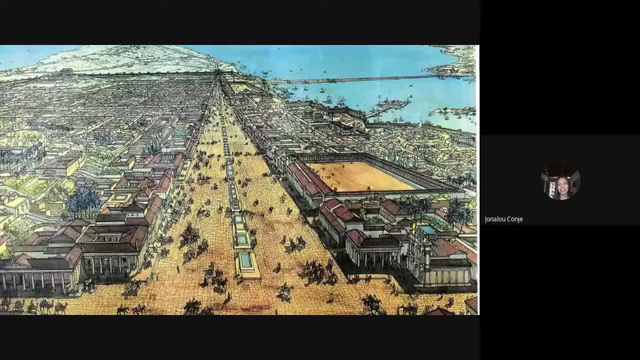 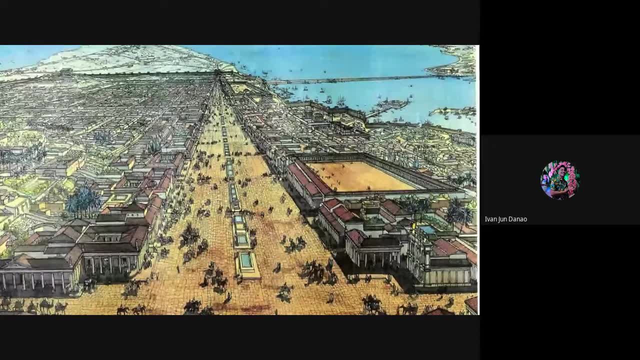 It is the city of Euclid who developed geometry. Okay, so that's more information that's intended. Now, the one that you're looking at is a city founded by no other than Alexander the Great, And the reason we're talking about it is because this is the city where Euclid has stayed most of his life. 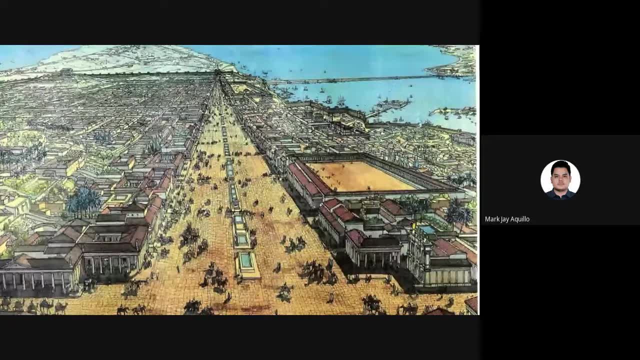 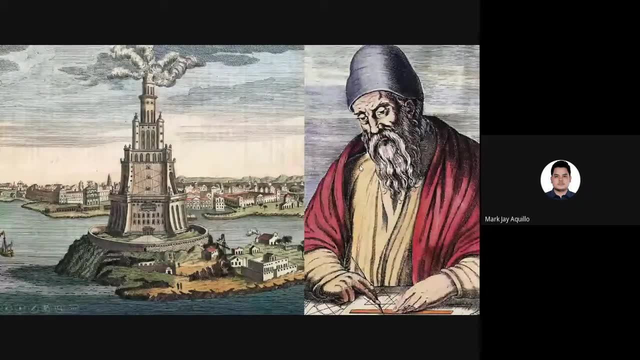 This city is famous for the Alexandrian Lighthouse, once then considered one of the wonders of the world and was destroyed along history. Most of the people of Alexandria nowadays petition for this lighthouse to be restored, But until now it has never been restored. 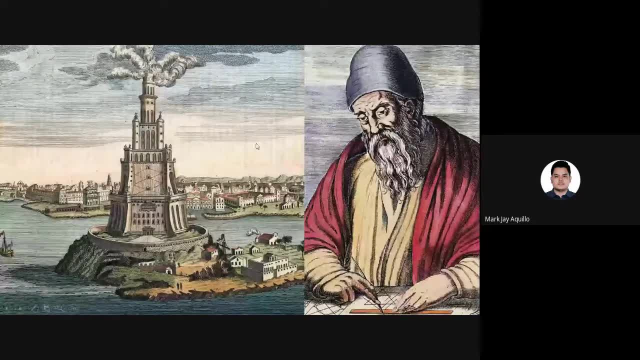 Maybe political reasons, We don't know. We're Filipinos, We're in the Philippines. Anyway, the one that you're looking at the right is the father of geometry. When we say geometry, we're mostly referring to classical geometry. This is Euclid of Alexandria. 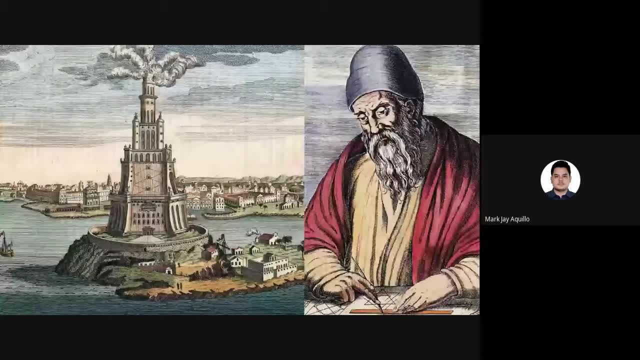 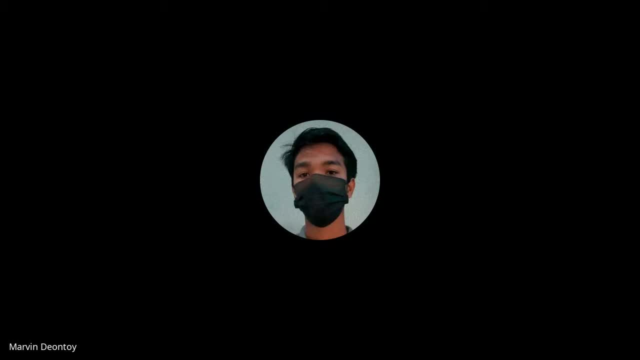 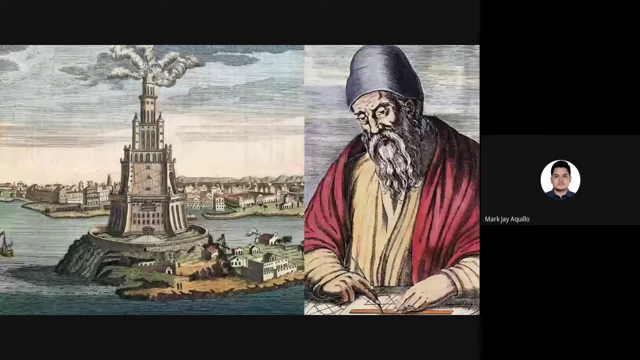 This needs to be Mathematician, while Euclid of Alexandria is the father of geometry. It's important that you know the difference, because it may appear as a question in the licensure examination for a teacher And you may get confused with Euclid of Megara, with Euclid of Alexandria. 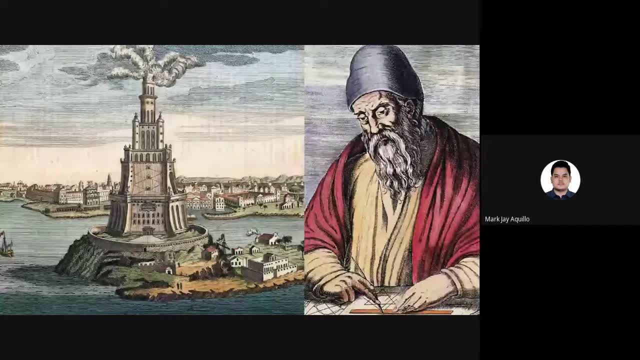 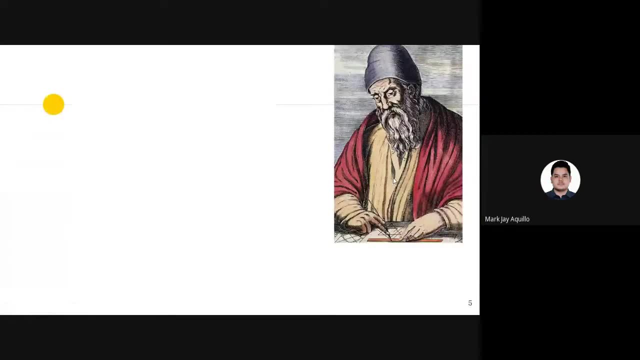 So you need to associate Euclid with the city of Alexandria? Sir, I don't know what to answer Now. you need to remember as well the famous work of Euclid. Who can remember the work of Euclid? Did you mention the name of the work of Euclid? 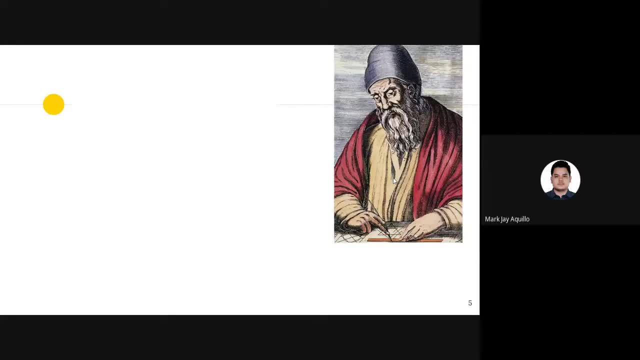 Yes, Of the work of Euclid before. No, sir, The only written one. the 13 books you said, Definitions, propositions, probability, Okay, So there's a name for that. The name of the work of Euclid I'm going to write on your screen is the elements. 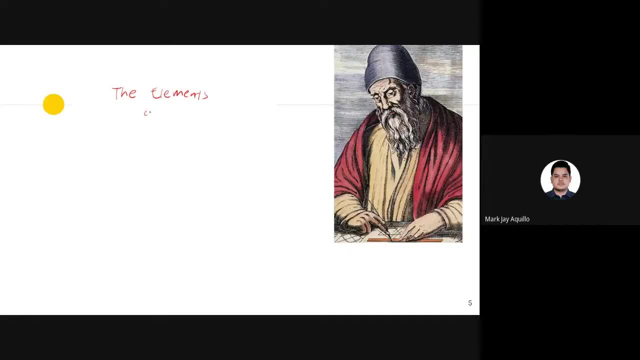 This is how he spelled geometry before geometry, But nowadays you're going to replace the IE with a Y And some people would only remember his work as the elements, But the full title of the work is the elements of geometry, Composed of treatises. 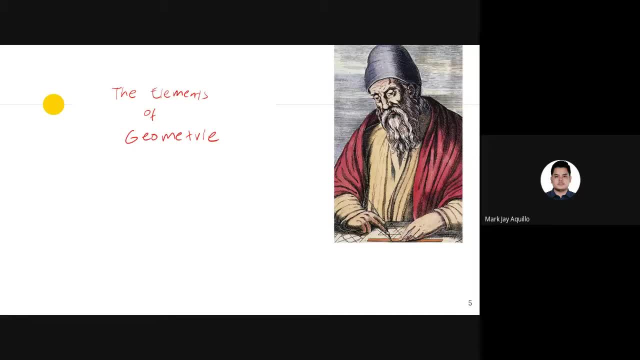 Proofs, Proofs, Proofs. Proven axioms in geometry. Now, who can remember Hello, Hello? Now, who can remember the number of books in the treatise, in the elements of geometry? Christian Joy, Yes. 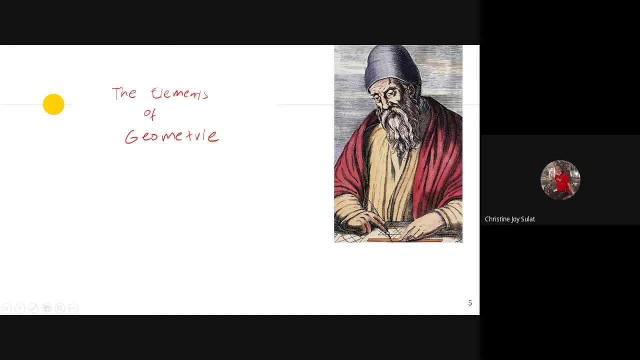 I think, sir, there are 13 books in the Treatise of Euclid of Alexandria. That's why he's called the father of geometry. Now, before we proceed, let's just explore this basic information that you need to know before we dig deeper into geometry. 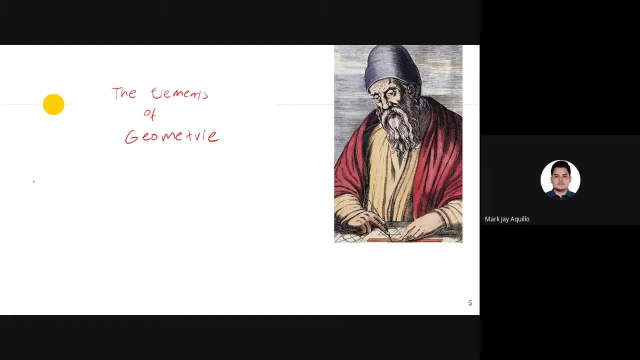 Geometry came from two roots. Who came first? Anyone, We have Ira, Yes, Ira. The first one is: G-U means earth. Very good, G-U means earth. The second one: Metri. Yes, sir. 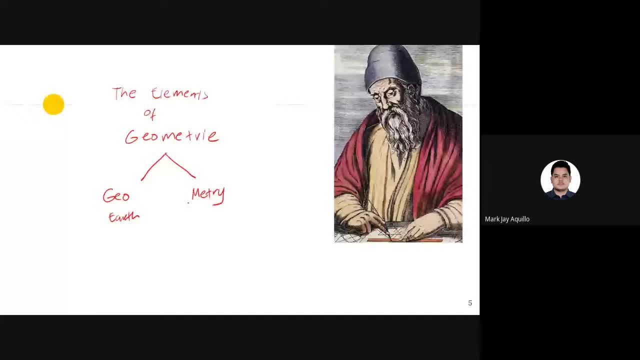 Yes, What's the second one? Metriforter, Metrifor Metrion, Which means Measurement, Measurement. Now, you need to remember this: The two roots of geometry is earth and matter, Because later on we're going to talk about them, when we talk about the life of one of 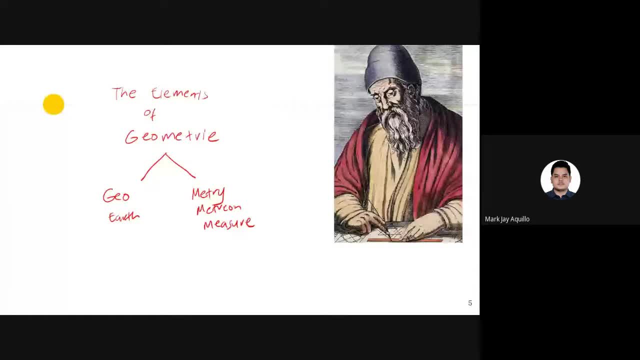 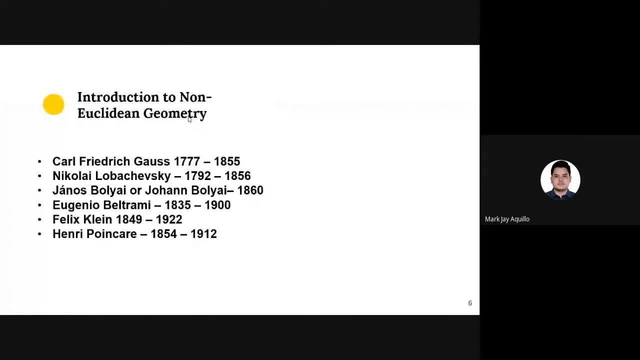 the mathematicians responsible for modern geometry. Let's talk about them. Modern geometry has been made possible because of the work of six mathematicians. Namely, we have Carl Friedrich Gauss, Nikolaj Lubaczewski, Yannos Boulier. 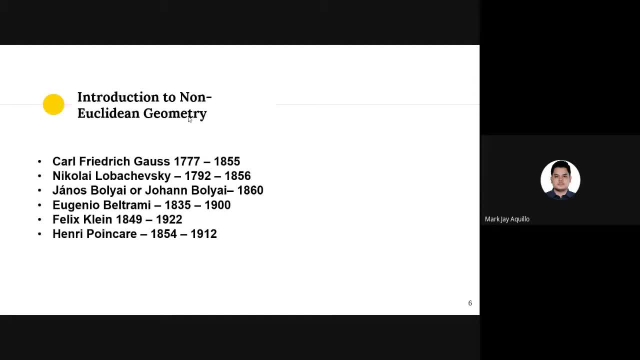 Yannos Boulier has another name. He's known also as Yohann Boulier, Eugenio Beltrami, Felix Klein and Henri Poincaré, a French mathematician. The first one that we're going to talk about is 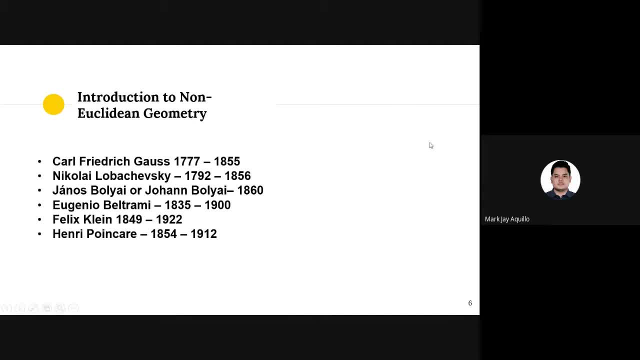 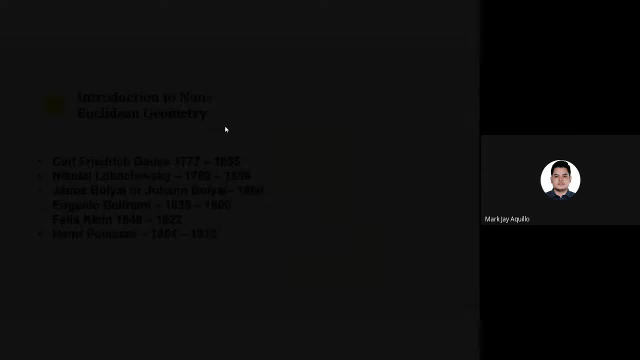 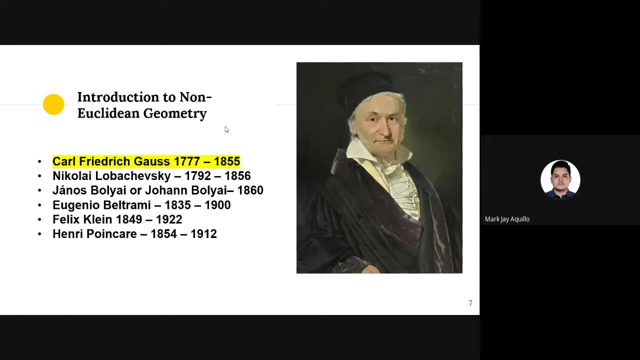 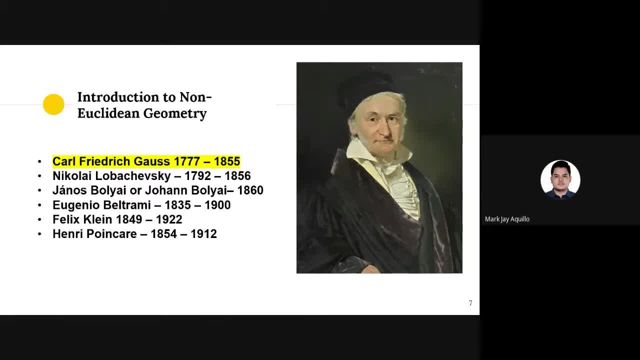 Carl Friedrich Gauss is you know what? he's actually the main player in this store. his work has made everything possible in modern geometry. he is a great mission from Germany and he's considered the preen kept mathematicorum, or the foremost of mathematicians, and he's considered the 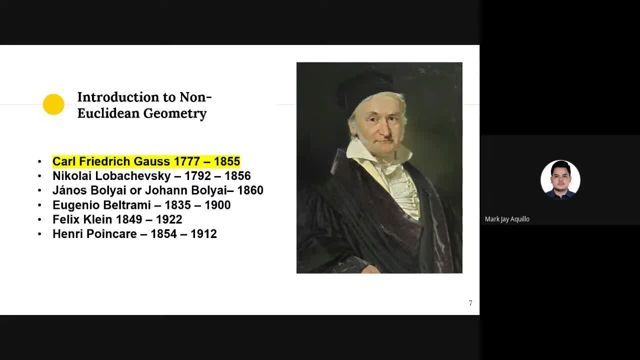 greatest mathematician since antiquity, whose importance for the world of mathematics is that he is the greatest mathematician since the 50th century, when one was to Accepted himself. he's one of the first Called, Only below Newton, or Code of barrels, only below Newton, Cocoa地. 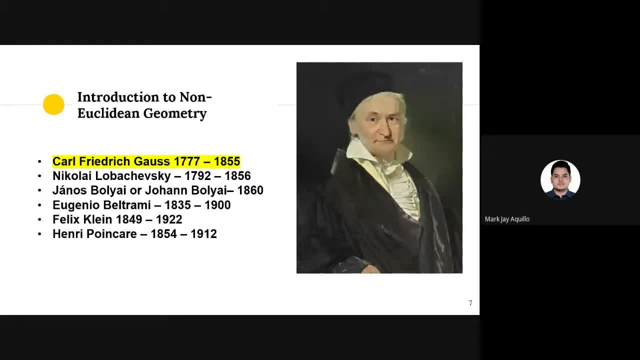 Called Only below Newton or Code of Car最後. calculate and Euler is one of most important persons in modern geometry. calculate and Euler is one of most important persons in modern geometry. cows was the dominant mathematician of cutting its spre shake changer. when we say 19 century were mostly referring to the age or the year. 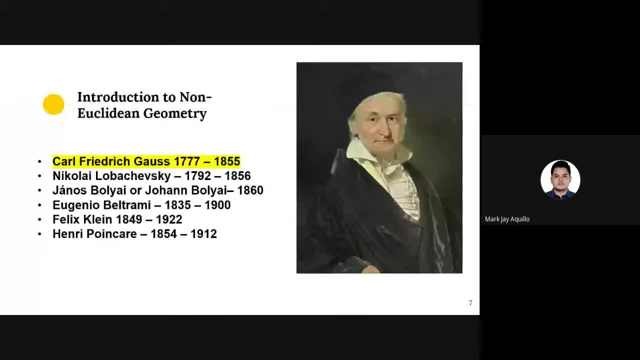 Güle G Break L. Mercedes G weil was the dominant mathematician of the 19th generic measure counting of 23 Gigabyte WiFi from United Kingdom. now I'll go to: I love this written letter W englandTV earlier in our earlier year when I e. 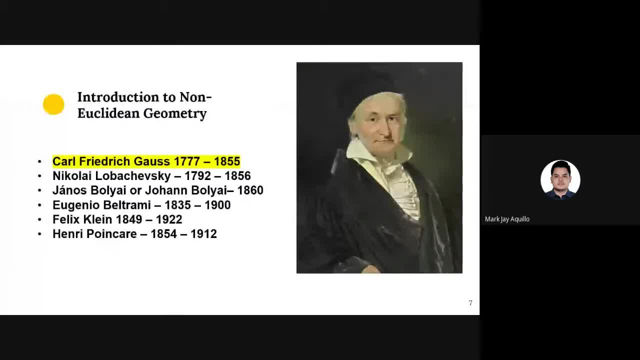 beginning from 1800 to 1899. That's 19th century, And he took the reins after Euler and Legrand. His work is mostly following the work of Euler and the work of Legrand And, as I mentioned before, he ranks only below Euler and Newton. 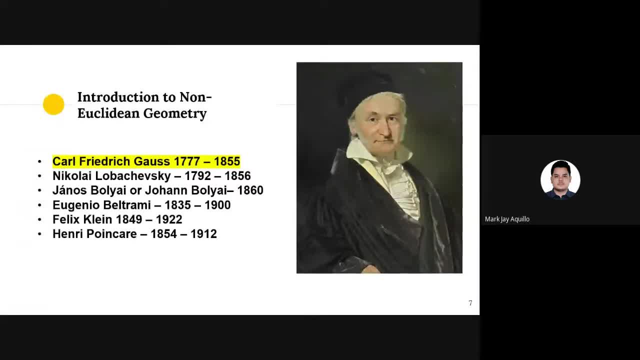 in the pantheon of mathematicians, He's one of the, you know, given a chance to go back to history. if you're really a serious mathematician, he's one of the mathematicians you're going to visit because at an early age he already demonstrated a keen sense for mathematics. 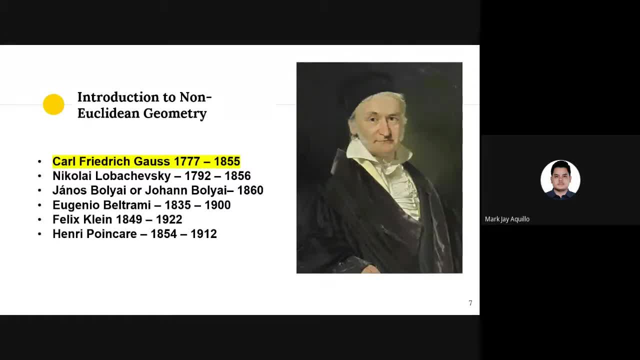 In fact, there's a movie made after him And, as a trivia, the name of the movie, if you're going to translate it in English, is To Measure the Earth. That's a play in the word, because he co-developed modern geometry. you know geometry. 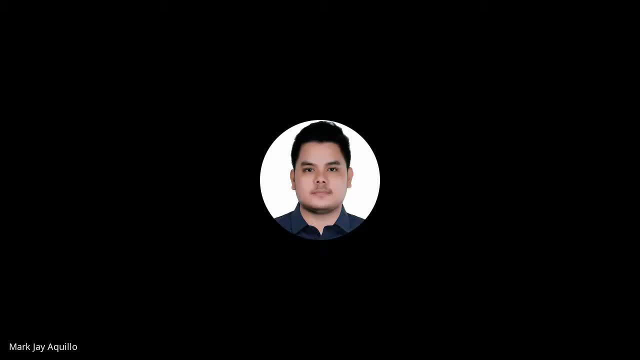 Earth measure And the title of his movie is To Measure the Earth. Now, the movie opened with a scene of him being one of the students in a class. I don't know, but they look like six to eight-year-old boys And there's a strict-looking teacher. 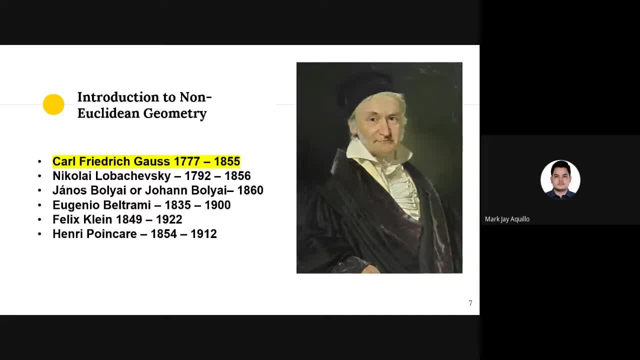 And in front, writing on the blackboard, a problem that they're supposed to solve, And, judging from the reaction of the children, it looks like there's a competition on who could answer the problem first. The problem goes like this: The teacher wrote 1 plus 2 plus 3 plus 4 plus 5 plus 6 plus 7.. 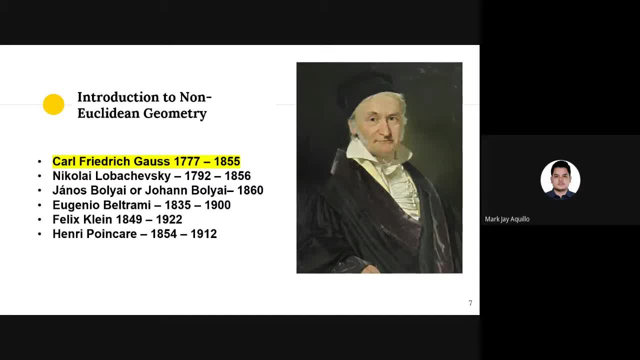 And then he told the class: do this until 100.. Now you know the usual response of the kids who want to answer it. first, they were all writing on a piece of what looked like a small version of a blackboard, a chalkboard, on their hands. 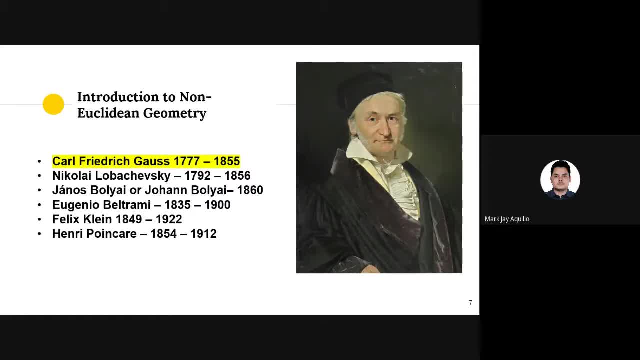 They're solving it and they're trying to come up to the sum, up to 100.. While Carl Frédéric Gauss was dreamily looking at the board not doing anything. He's not even solving, And what happened is one moment. I need to pause this. 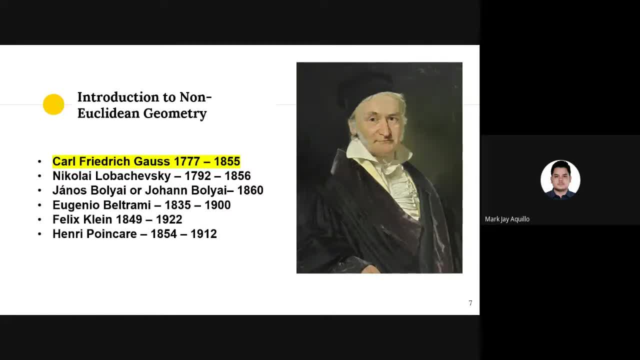 One moment I'll go back to some some someone important came. They've taught me that it's less to call for yourself to once you've heard your name. it's way more time to go here than back home just when you've been thinking. 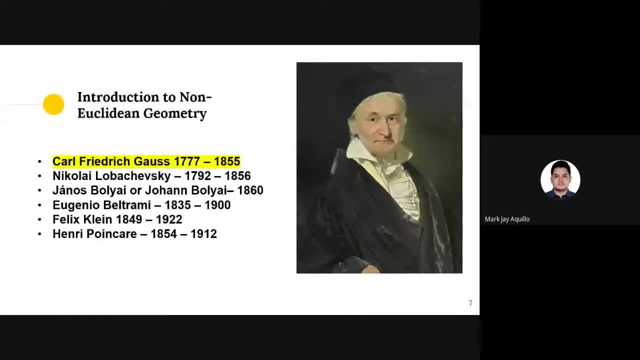 I juste want to fall back in shape. Haha, you're making the lot more difficult, so you'll have to do that. You don't have to. Human beings don't have enough energy. okay, going back now, carl frederick gauss, as a kid, was dreamily looking at the board. 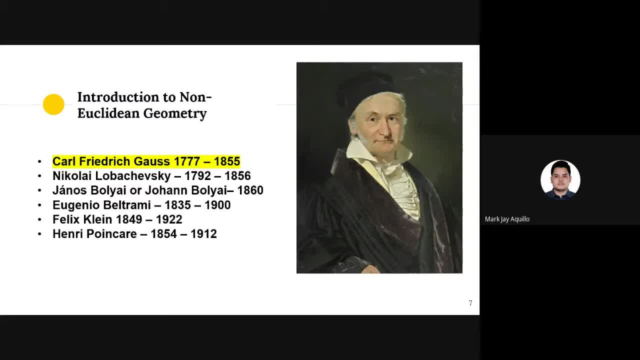 and the teacher was a bit not happy about it. minutes after carl began writing on his own board and after a few seconds perhaps, or a few minutes, he is ready with answer. he gave it to the teacher and the teacher was dumbstruck. he was angry because he was thinking carl was cheating. 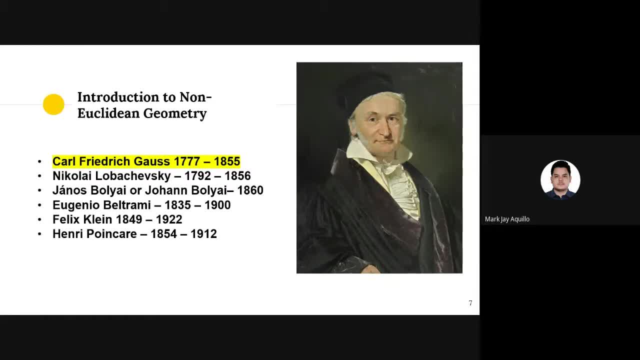 so he asked carl what he did and he demonstrated it in the board. what he did is he wrote the numbers four word first: one, two, three, four, five, six, seven, and on the second line he wrote it backward: one hundred ninety nine, ninety eight, ninety seven, ninety six, something like that. 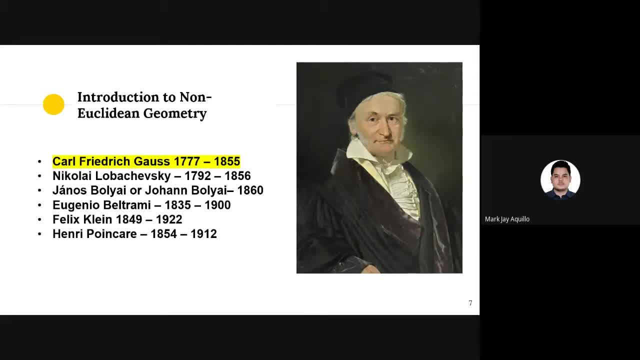 you and he demonstrated that, the sum. he demonstrated that the sum of each of the peers is always one hundred, all throughout. you know the, the number of life. so postulated, there must be one hundred sums of one hundred one hundred to get the sum. since you wrote the lines, he divided it into two. 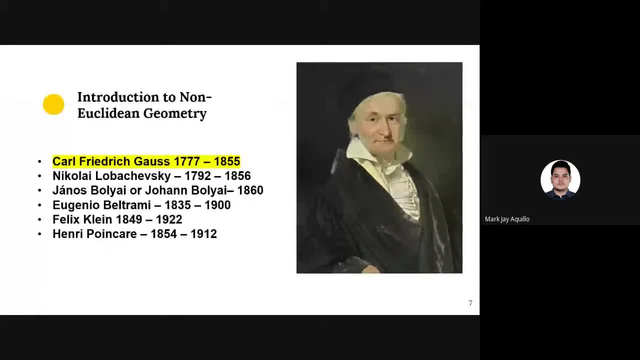 giving him five thousand fifty, and he was correct and is actually the origin of such a method appeared. okay, let's proceed. so that's carl free gals and that's what we can do: lessons. it was a trial. now, if someone of you has given us thought about that, 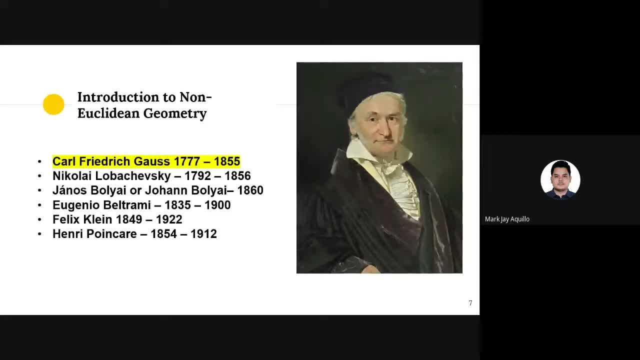 like, if you want to add numbers forward consecutively on a rhythmic sequence or something like that, and that the way to do that is to just write the numbers backward on the second line and add them up and multiply by the number of terms and divide by two, then you must be as great as Kyle Friedrich Gauss. 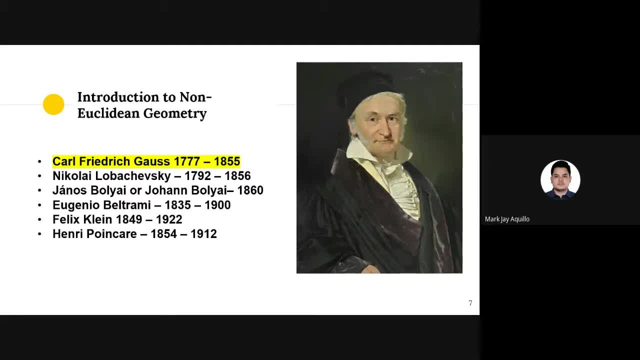 You must have the potential. You just inform us and we'll nourish it further. Now, what happened is when he grew up. you know, during his time everybody was obsessed with the fifth postulate of Euclid. Euclid has five postulates. 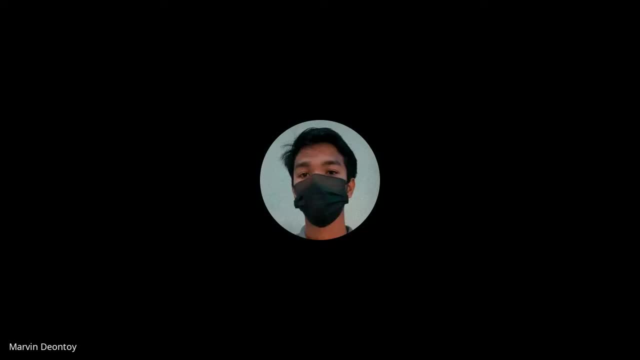 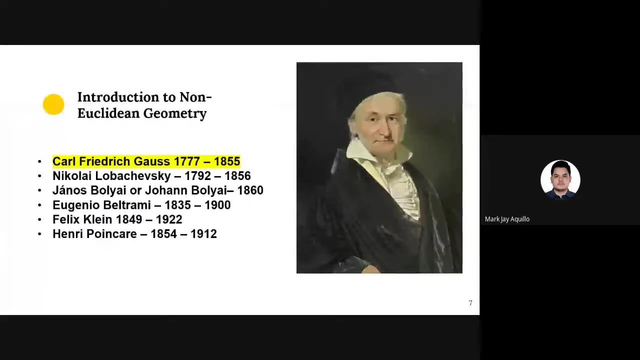 Sir, Sir, nawara Nawara po sir. Yeah, I know I'm still here Going back During his time, during the time of Kyle Friedrich Gauss, people were trying to prove the fifth postulate of Euclid. 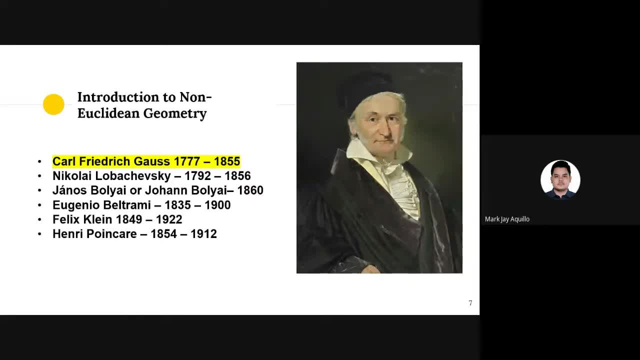 The fifth postulate of Euclid was one of the five postulates And they were trying to prove the fifth using the other four. Okay, So that was the work. How did they do it? Remember how you did: proving in logic and set theory. 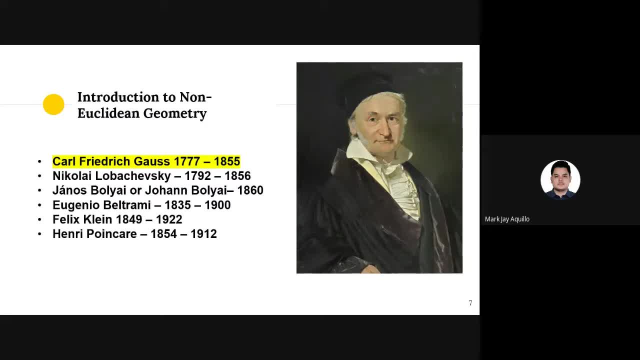 That's the same thing. You're trying to arrive on the fifth postulate by beginning on either of the four and using the rest of the four as probably your middle line From then on. Gauss already knew that there's modern geometry. He has already worked on modern geometry. 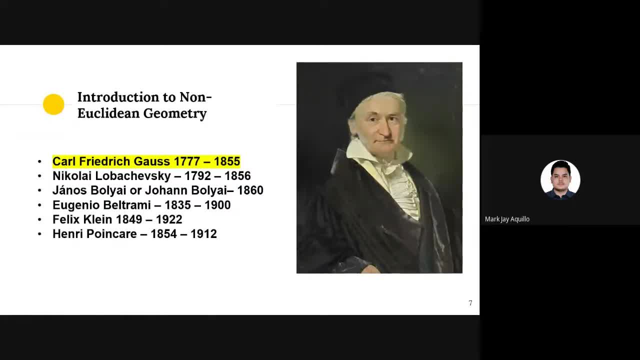 He has written his paper, but during his time no one would believe him. It's like the time of Galileo: No one would believe that the earth is, that the sun is the center of the solar system, Earth was. That's a predominant belief. 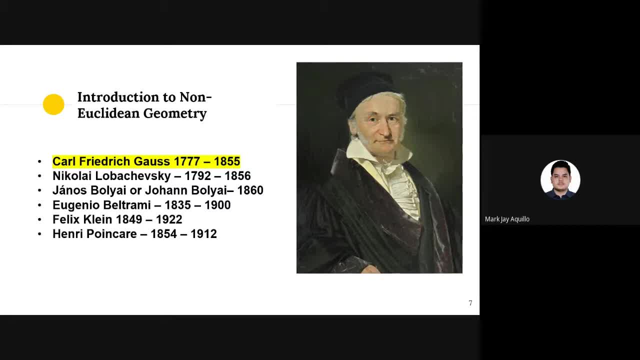 And what happened to Galileo when he put forward the idea that the sun is the center of the solar system? He was ostracized. so he doesn't want to offend everyone, He doesn't want to go against the common knowledge of his time. 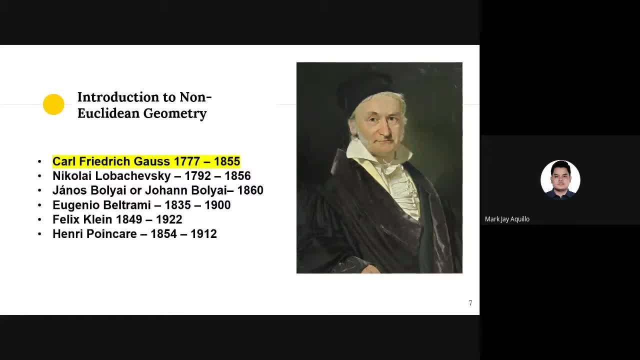 What he did because he was reluctant. he kept his paper. He kept his paper and research to himself and never published it. That was during the 1800s. Now, years after, there are two great mathematicians in the name of Lobachevsky and Bollier. 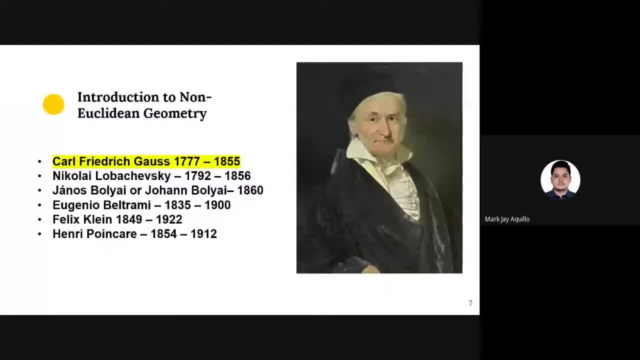 Lobachevsky was a Russian mathematician and Bollier was Hungarian mathematician. Now the three of them I need to punctuate. first, Gauss was German, Lobachevsky was Russian and Bollier was Hungarian, Although Russia is partly Asia, if you notice the three foremost people who founded modern. 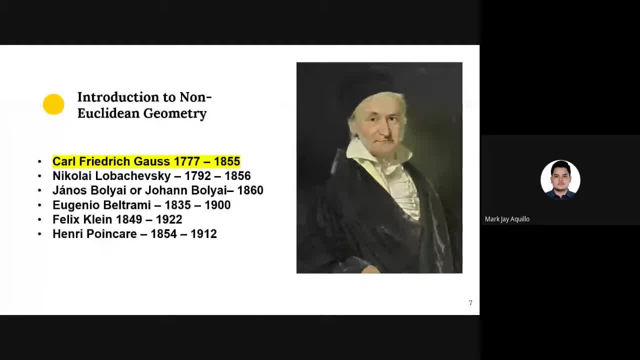 geometry are all European, of European descent. Now, after years, Lobachevsky in Russia and Bollier in Hungary independently discovered modern geometry around Earth In 1830, of the two, though, Lobachevsky was the first, And while they were finishing their paper they were trying to publish, it became clear. 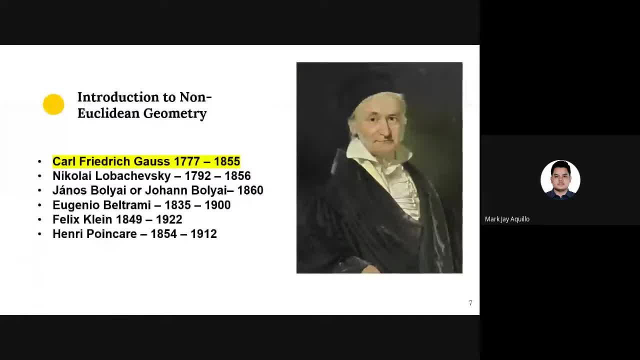 to them that Gauss already discovered it years ahead of them. This was the story of that Janus Bollier had a father, Wolfgang Bollier, And, like many mathematicians before, Wolfgang Bollier had a father Wolfgang Bollier, And like many mathematicians before, Wolfgang Bollier had a father Wolfgang Bollier had. 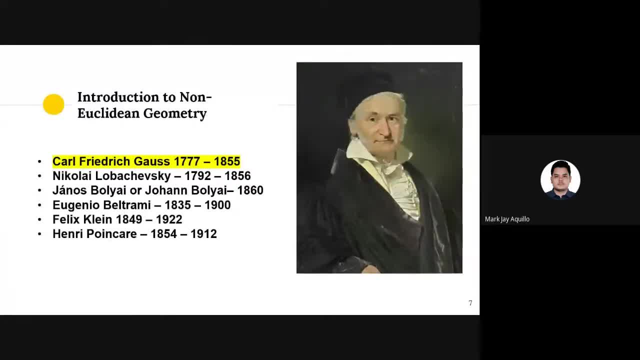 a father, Wolfgang Bollier, And Wolfgang Bollier had a father, Wolfgang Bollier. Wolfgang Bollier also worked on the fifth postulate, Wolfgang, because during those times there are a few mathematicians and academicians befriend themselves like mathematicians befriend other mathematicians to extend his 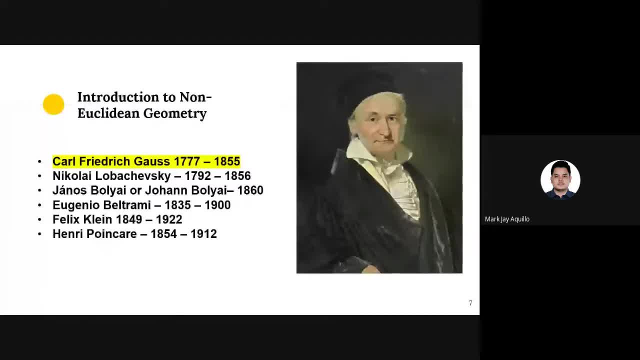 network and his knowledge. So Wolfgang is a friend of Gauss And for years. Here is Wolfgang Bollier. Here is Wolfgang Bollier. he has tried to discourage Janus Bollier. According to him, stop working on the work of Euclid anymore. 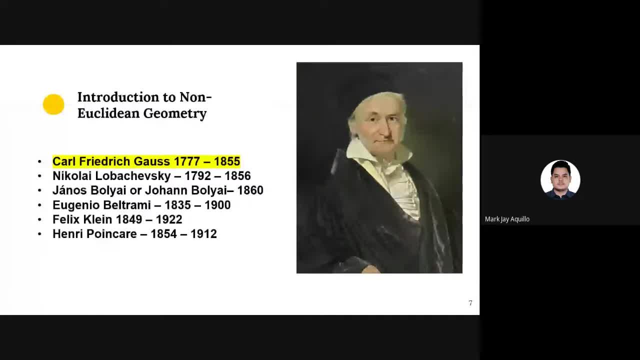 because I've wasted my time doing it and I amounted it to nothing. But Janus Bollier, being obstinate, himself worked on the fifth postulate and in the process he discovered modern geometry. He wrote a paper on it and Wolfgang, being a proud father, told Gauss about it. 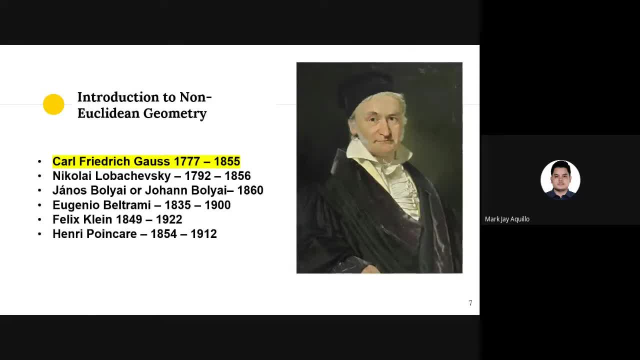 And he said- it's not really the exact words, but probably he said: Hey, Gauss, you know what my son is so great. he developed a different type of mathematics. It's called modern geometry. And Gauss said confidently: modern geometry. 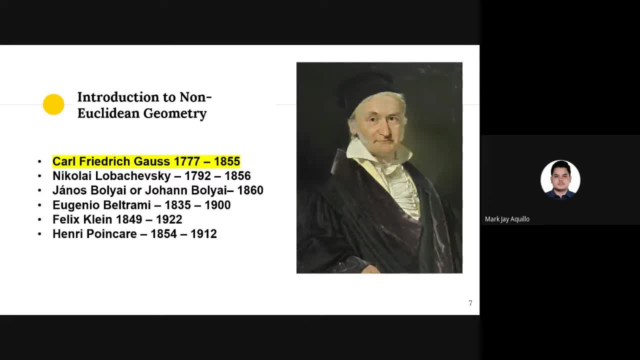 I already know everything about it. Many years ago, when Janus Bollier found about it, he was so frustrated he stopped pursuing the work. He was frustrated because he thought all along he was working on something original, and only to find out in the end that it's just a work that was already finished by Carl Friedrich Gauss. 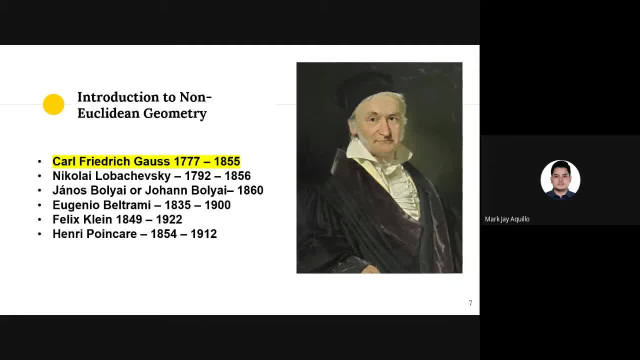 But in his small town, you know, while Bollier has already been discouraged, Lubashevsky was doing his work. He finished his work and Gauss heard about it. Gauss became so curious about the work of Lubashevsky on modern geometry. 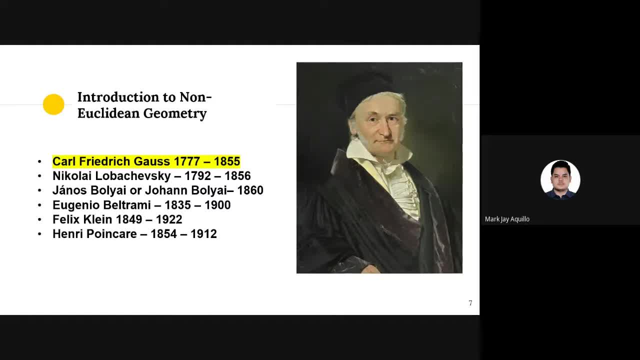 that he purposely- according to the story, he purposely- learned Hungarian just to understand The modern geometry take of Lubashevsky. Now, before we proceed, because we've been mentioning about the five postulates of Euclid already, let's talk about them first. 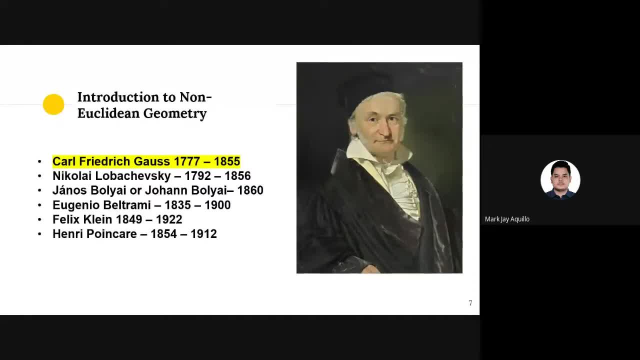 It will be instrumental in your learning of modern geometry if you'd be able to understand them as early as now. Now the first. So what I'm going to do with the postulates is I'm going to simplify them, give you an equivalent of the statement that we would be able to learn in one sitting. 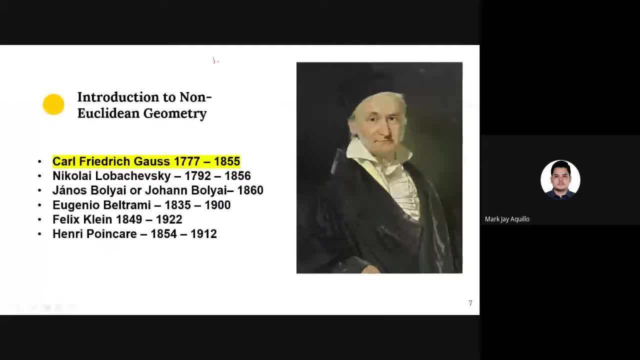 But along the process, because the five postulates are so important in your journey for understanding modern geometry, we're going to dig deeper into them in details, In their original statement. Now, the first postulate says that if you have two points, I'm going to draw two points here. 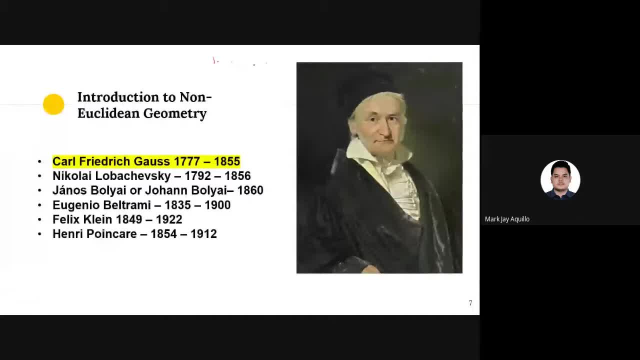 Let's say you have two points in a surface, According to Euclid, you can always draw a unique line between them. So here, So whenever you have two points, you can always connect them To create a unique line between them. When we say unique line, it means there is only one line that could connect two points in a uniform field or plane or space. 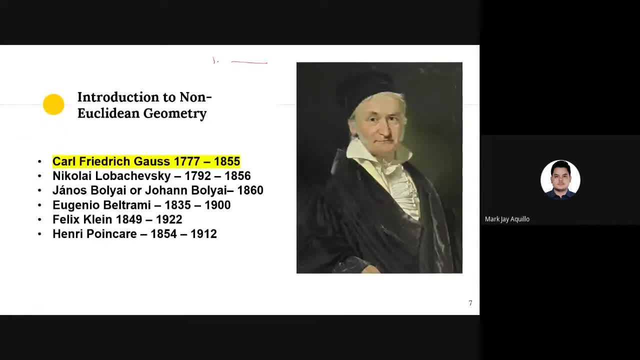 Again. the first statement is there's only one line that connects two points. The second postulate states that if you have a line, it sounds more like an extension of the first. If you have a line, you can always extend them both sides indefinitely. 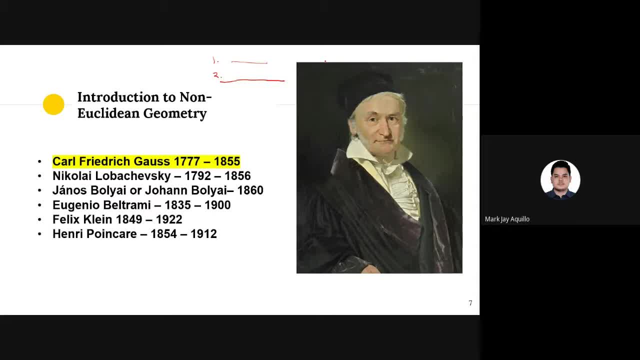 That supports the statement that a line extends both sides infinitely. That's the definition of the line, by the way. So whenever you have a line, however big or small, you can always extend it on either side. The third statement. Now, you must be wondering by now. 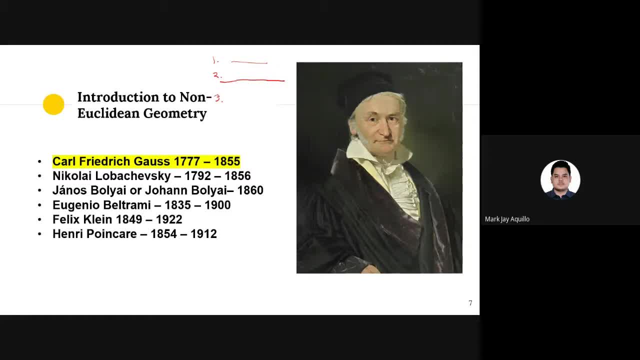 why are these statements simplistic and obvious? That's the point. These five statements are axiomic in nature. You don't need formal proof to prove them, Because they're so obvious. you can easily spot that they're true, Unless you use a different type of geometry to disprove them. 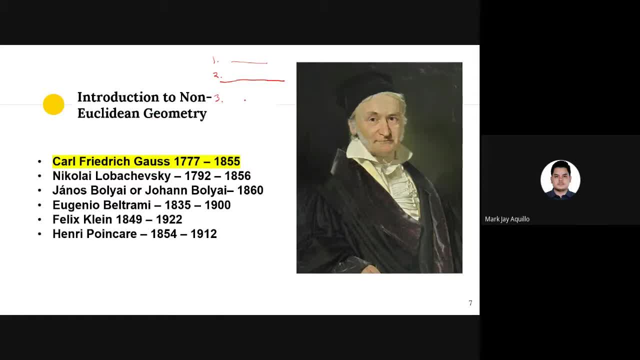 The third statement is: if you have a and a radius, you can always create a unique circle. That means, if your radius is 3,, the circle that you could create is unique to that, if your radius is 4, and so on and so forth. 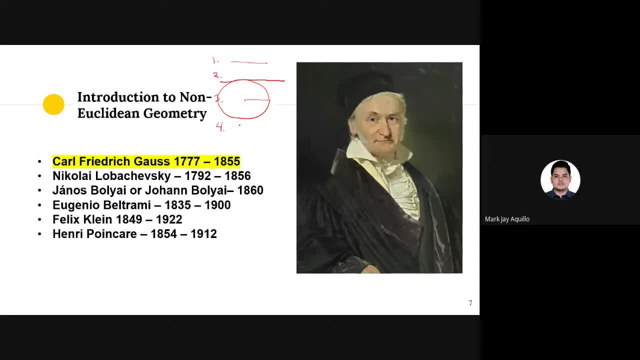 The fourth statement states that all right angles are congruent, Essentially the same. So the right angle in Ira's place is literally the same as the right angle in Katrina's place. If Ira is going to try to measure it, it will be 90 degrees. 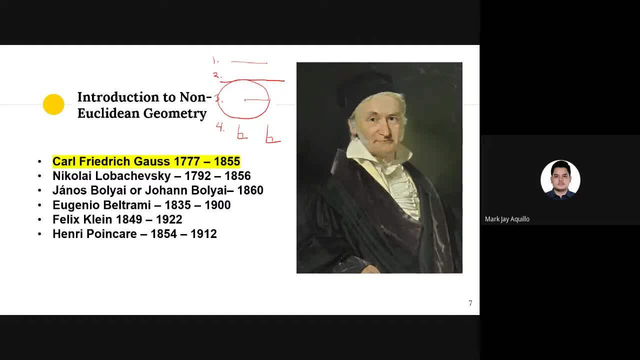 And if Katrina wants to validate it, it will be 90 degrees. In all essentiality, they're the same. Now, the fifth and the most controversial of these postulates states that if you have a line and if you have a point away from the line, 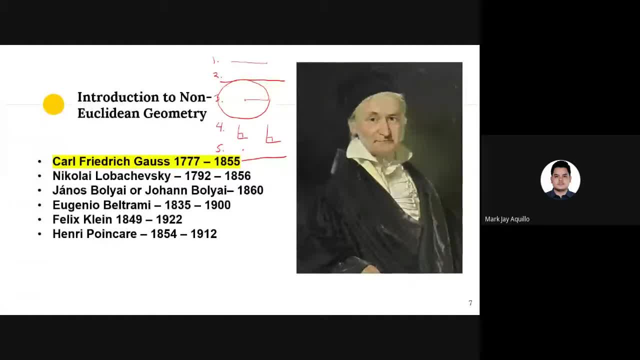 the reason we're saying away from the line is because the line is a collection of points, So it must be outside the line. If you have a line and a point outside the line, then there is only one line that you could draw that is parallel to that line. 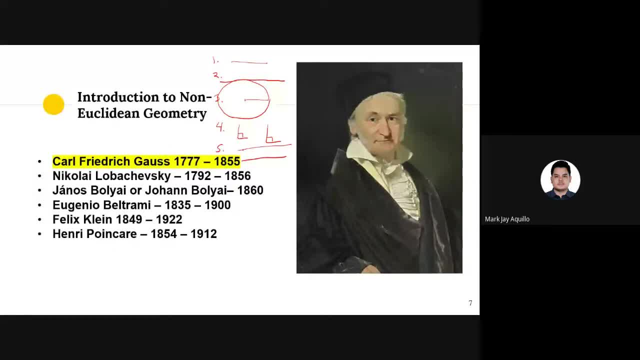 Or we could say: if you have point A and line L, then you could only draw one line through point A, parallel to line L. When we say parallel a line, that will not meet or intersect with line L, even if we extend the line on both sides indefinitely. 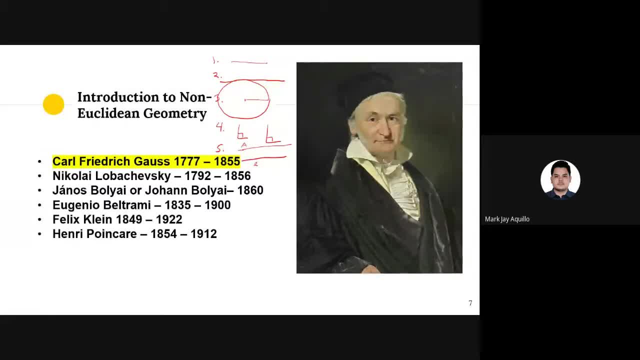 That's basically the definition of what's parallel And over the course of the work these mathematicians have tried to prove that there is only one line that could extend. I mean that one could draw that is parallel on the other line Along the way. 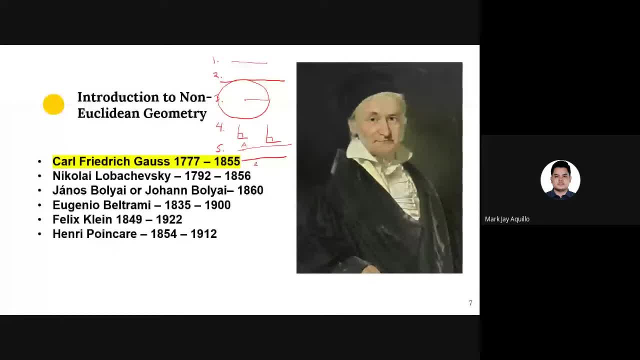 these mathematicians, Carl Friedrich Gauss, Nikolai Lobachevsky and Yanis Bollier, in their investigation found out that on a different situation, there could be infinitely many lines that you could draw that is parallel or non-intersecting with that line. 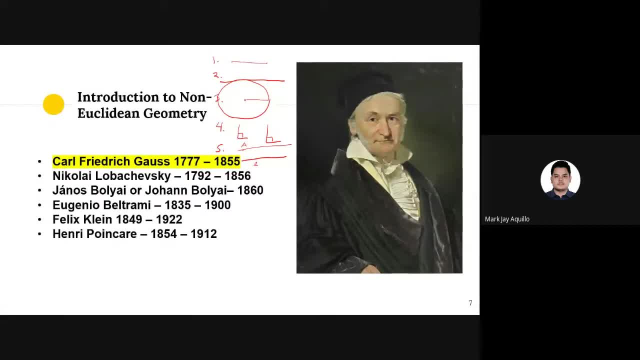 especially if your geometry is non-uniform geometry. And that paved the way. the efforts of these mathematicians to prove or otherwise discovering that it can be disproved by a different type of mathematics paved the way to the discovery of modern geometry. Now, 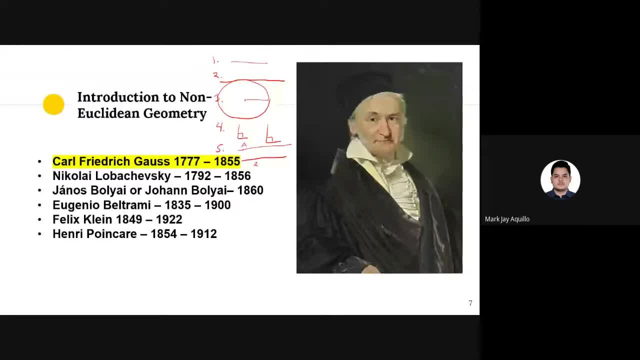 let's go back to the first question. Gauss realized, while trying to prove, while trying to attempt, while attempting to prove the fifth postulate from the other four, that there could be a different geometry, like Euclid, but might not be a line through a point that doesn't meet a line. 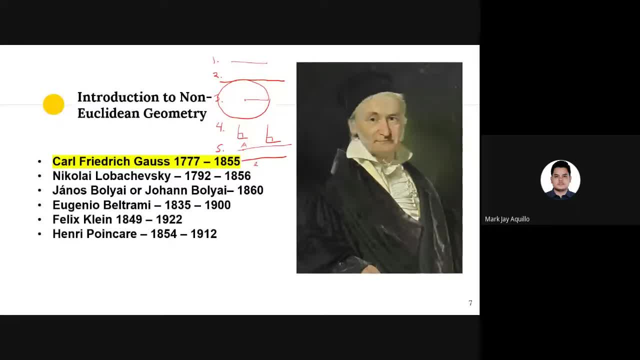 So it's like Euclid, but it's different. It was unclear first in the work of Bollier-Lubachevsky, but Gauss started developing this geometry. That geometry that was essentially discovered by Gauss was the geometry in the surface of a sphere. 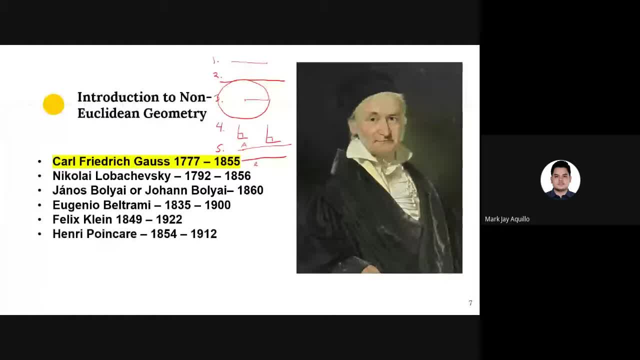 or what we call the spherical geometry. And if you're going to notice spherical geometry, if I'm going to draw a sphere here, notice that in the sphere all of the elements of a classical geometry can be demonstrated in a sphere, For instance, 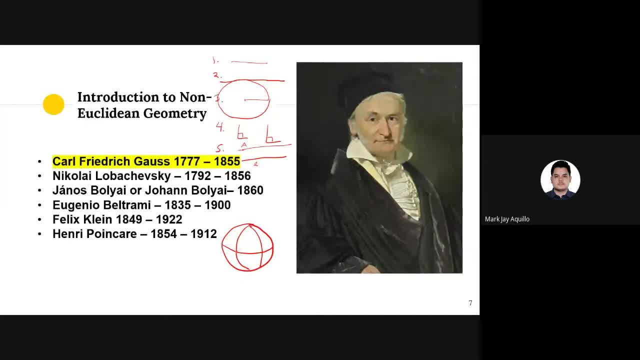 there is a point, a point on the surface of a sphere. that could also be the same point as that of a uniform plane. There's also a line, but in the definition of a line in modern geometry, particularly in spherical geometry, a line is called a great circle. 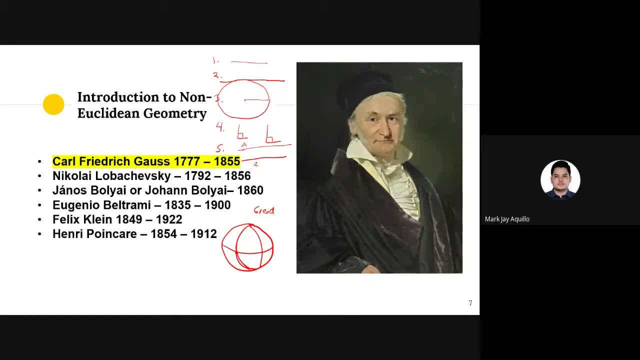 and it doesn't extend indefinitely. It ends because it has limits as to how much it could extend. Basically, it's a circle. It's like if you're going to cut a plane through a sphere, If I'm going to cut it here. 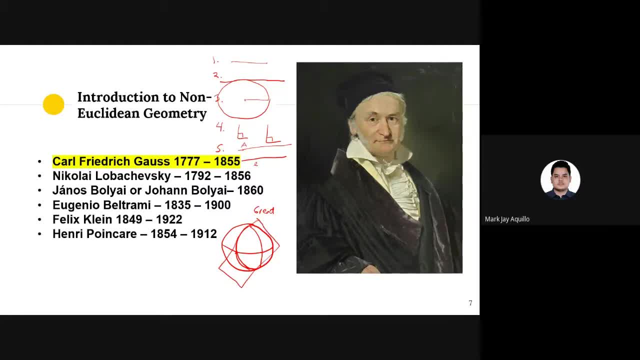 let's say you force a plane through a sphere, you're going to form a circle. That's basically a line, Remember a globe, where it has longitudes and latitudes. These are the lines on the surface of a sphere. But if we're going to extend them further, 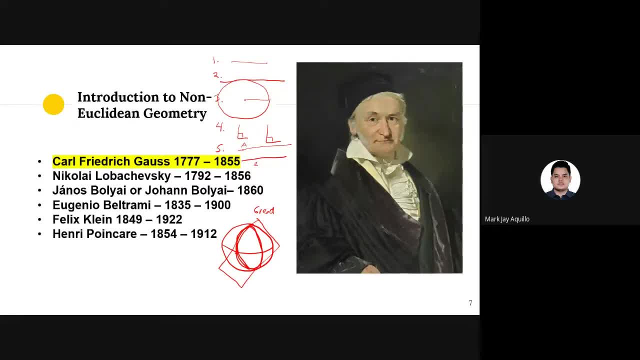 you'd notice that you'd go back to your point of origin, thus giving you a circle instead. In the mathematics of spherical geometry, a line is called a geodesic. It's basically a curved line forming a great circle. There's also angle in a sphere. 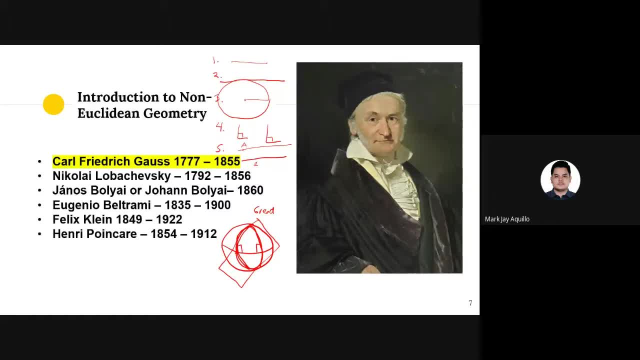 But the angles formed on the surface of a sphere follows a different rule than that of a regular plane. For instance, the triangle that can be formed on the surface of a sphere may exceed a sum of 180 degrees. It could be a positive curvature triangle. 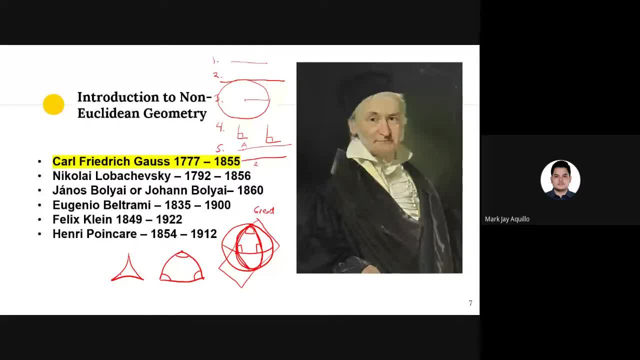 or a negative curvature triangle, as opposed to the regular triangle of a plane. Now, these positive curvature and negative curvature triangles, we call them geodesic triangles because their sides are geodesic. They're very telling. property is the sum of their internal angles. 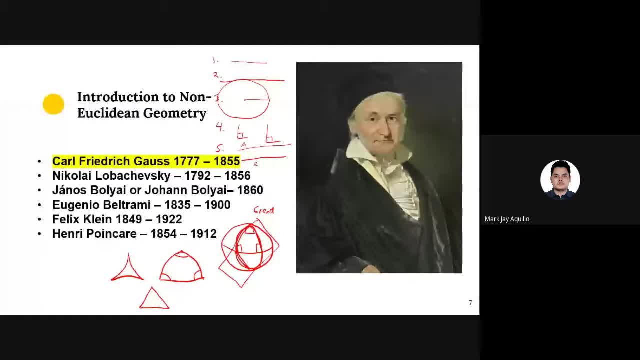 exceed 180 degrees, Or it could even be less than 90 degrees in the case of negative curvature triangle. Now, Lubashevsky and Bollier worked on the same geometry at the same time. Lubashevsky was ahead of Bollier, though. 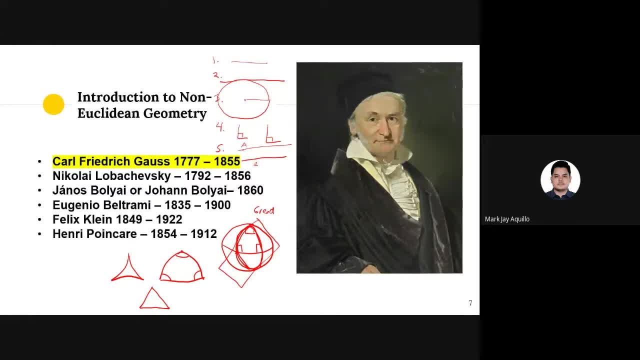 And Bollier was discouraged because he found out that Carl Friedrich Gauss knows about it, But of the three of them, only Lubashevsky was able to publish it. It's probably one of the many failures, I mean one of the most significant. 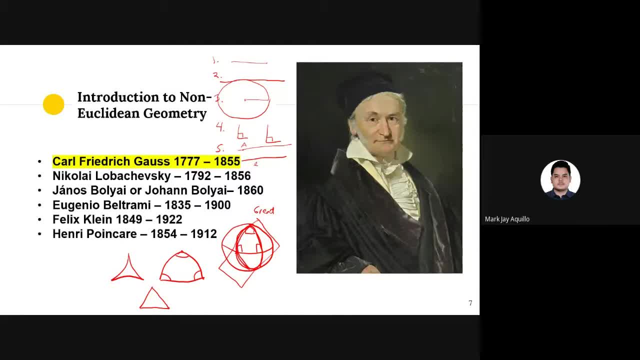 failure of Gauss because he was reluctant. He doesn't want to frustrate other mathematicians, so much so that he did not publish his work. Somebody else did, And that's Lubashevsky, years after Gauss found about it, Aside from Okay. so I'm going to show you the faces. 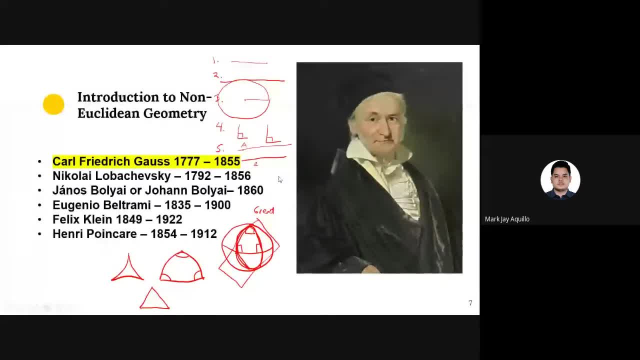 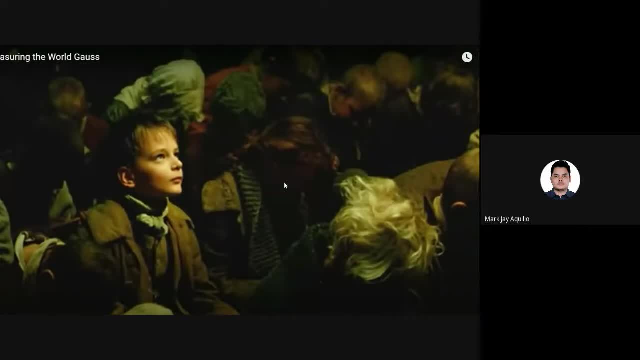 of these famous people who have been talking without showing their faces. This is a. this is the introductory video of the German movie To Measure the Earth about Gauss. If we're having face-to-face class now, this is a movie time. You know, we usually watch. 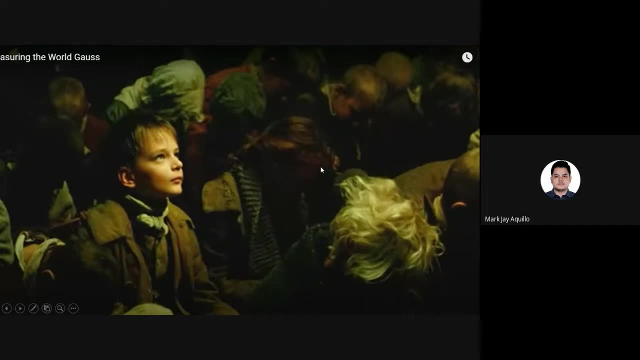 this movie as part of the class, But sadly I cannot compel you all to watch the movie because it would consume a lot of your data. So instead of I don't know, maybe I'm going to share with you the link. Let me know via the. 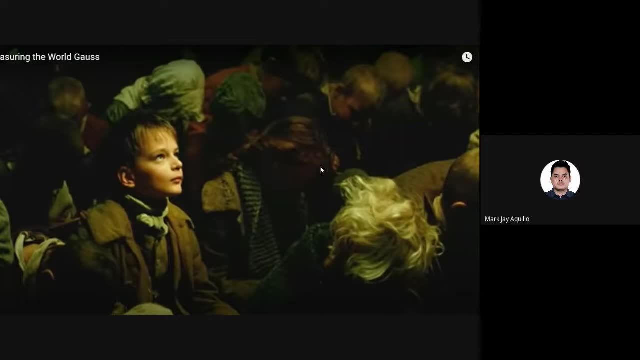 in-call messages. if it's necessary for me to share the video via the Google Class- Either the video or the link- Because I'm going to do it if you ask, so that some of you could, you know, probably get entertained with the life of. 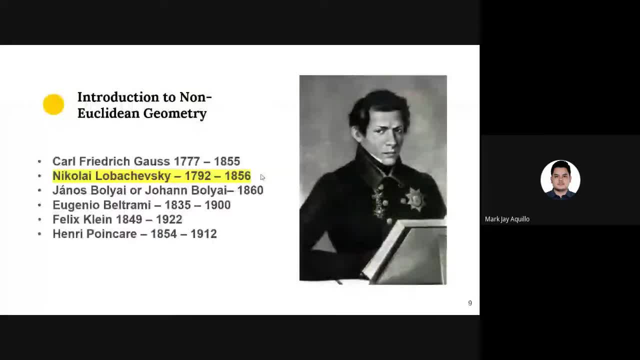 Frederic Gauss. This one is Nikolai Lubashevsky. Look at him. He looks very angry. in the picture He looks very negative. He grew up in a poor town in Hungary And he grew up mostly poor, But he was intelligent. 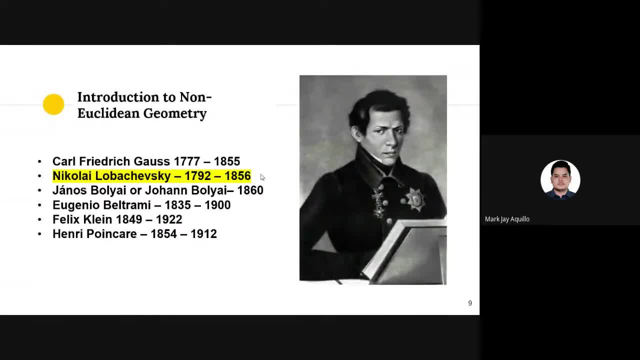 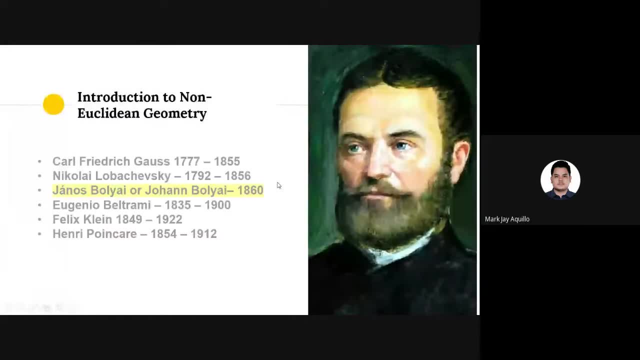 And he did not learn English or German, So Carl Frederic Gauss learned his language in order to understand his work. instead, This is the frustrated Janus or Johann Bollier, Son of Wolfgang. Wolfgang is the inspiration of the famous software Mathematica. Mathematica is the best. 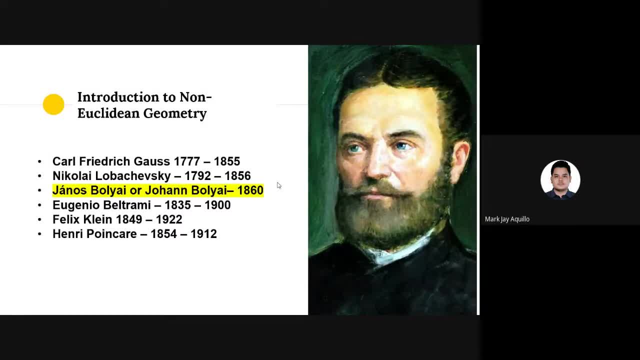 software if we're going to, if we're going to do computation or graphing in mathematics, Only that while it's very powerful, it's also not free and it's expensive. So for mathematicians we contend ourselves to with the cheaper software, Mathcad or GeoGebra. 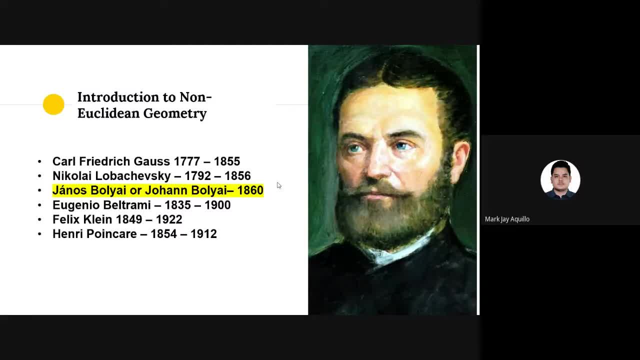 But if you have the money and if you want visualization that's powerful, that enables you to do Python programming. you do Mathematica Now. before we had a technology- mathematical teaching- and we learned about it, but the curriculum changed and you know Okay. so those are the three famous 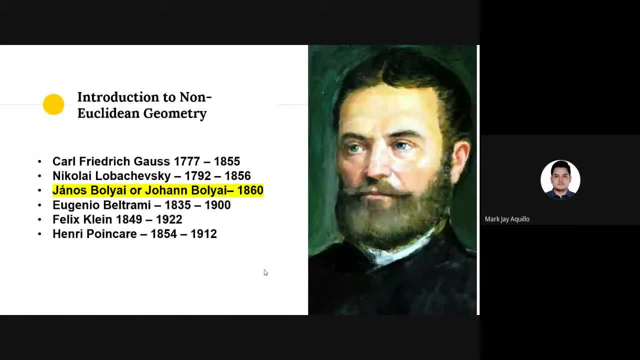 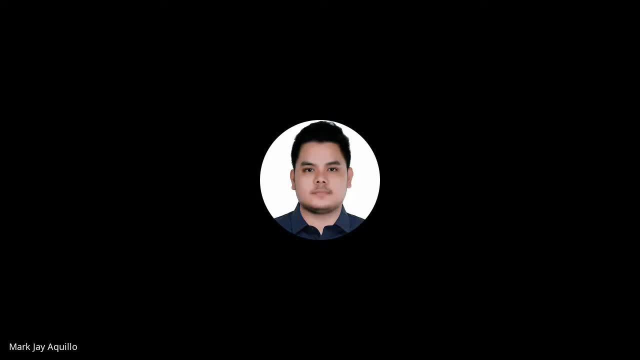 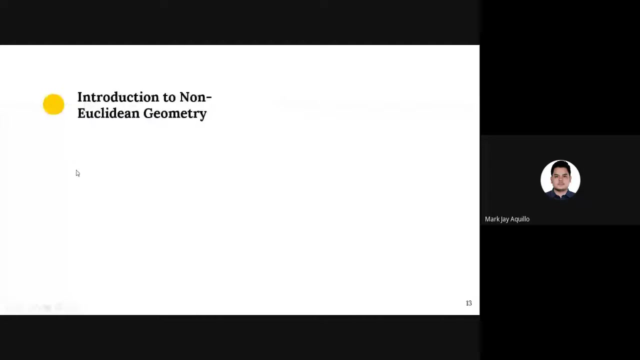 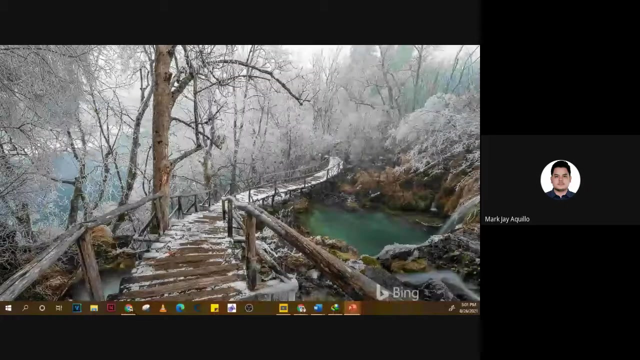 people that we just talked about. The rest, we have Eugenio Beltrami, Italian also. I lost. Okay, so did you see? Eugenio Eugenio Beltrami, Eugenio Beltrami. Eugenio Beltrami is Italian here. 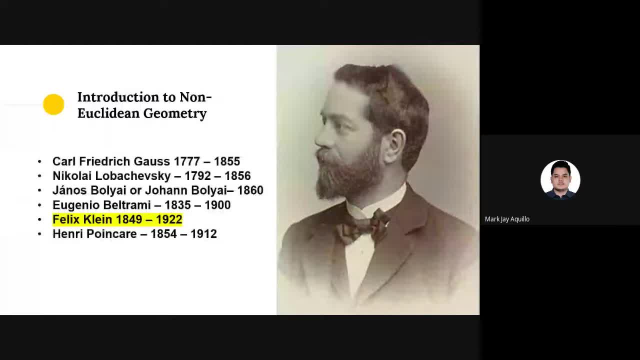 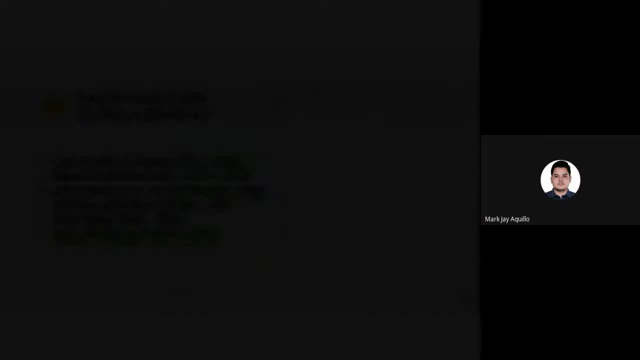 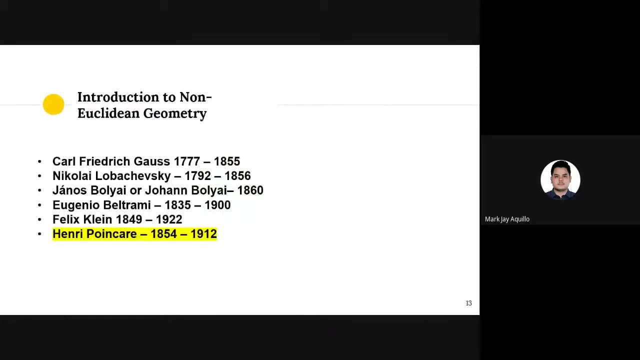 And the next one is: we have Felix Klein, I think it's German, And the last mathematician is- I don't have a picture, I'm sorry. maybe you can reach for the picture. The last one is a French mathematician. his name is. lucky for you. we're having 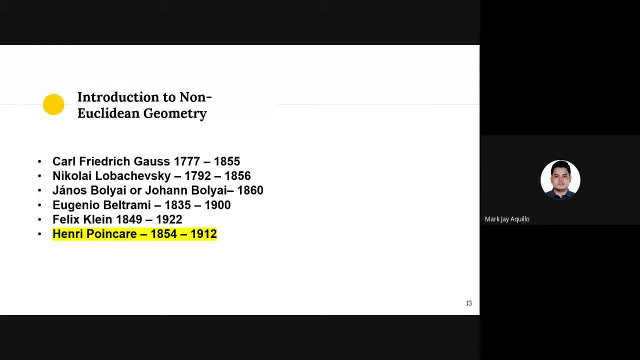 French class and the correct pronunciation of this: Henri Poincaré, Henri Poincaré, Henri Poincaré, not Henri Poincare, that's. you know that's a wrong way of pronouncing it, Henri Poincaré. The three of them worked. 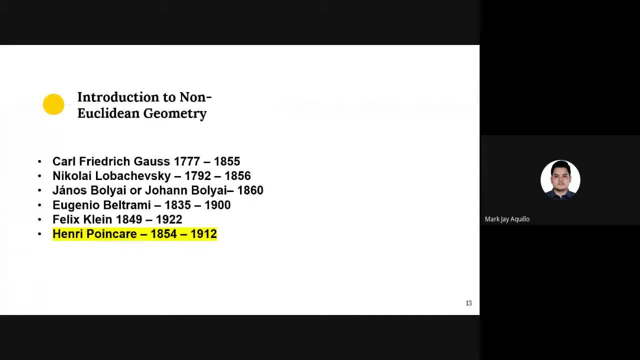 by extending the works of Carl von Friedrich Gauss, Nikolai Lobachevsky and Janus Bollier. Now, from the spherical geometry, other geometries that are non-Euclidean arose. By the way, some mathematicians remark how frustrating it is that for the past thousands 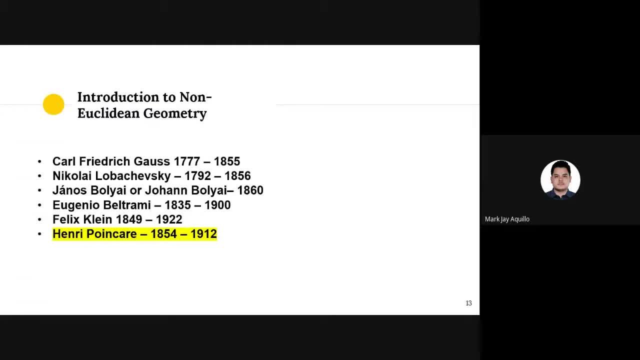 of years we have been studying spherical geometry, but we did not realize that it's a mathematics distinct from Euclid. You know, Ptolemy studied the heavens when he studied the planets, the heavenly bodies, and if you're going to look at the sky, literally, 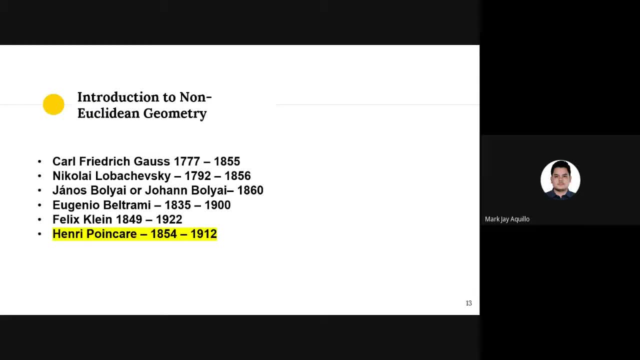 the sky is spherical in nature. it's like a surface of a sphere, but this time you're looking from the inside and basically what they're doing is they did measurements, they did mathematics to approximate the distance of one object to another, and that's basically spherical geometry. 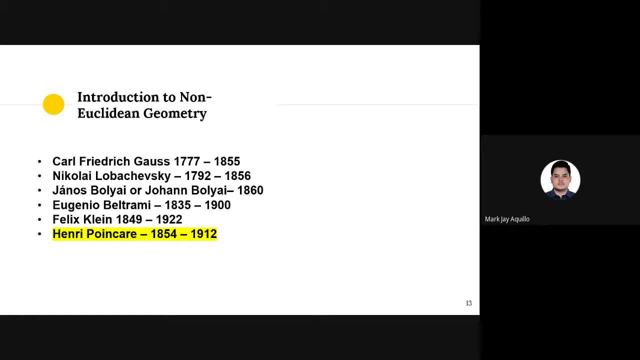 in this course, given that we are under pandemic and given the difficulty of studying everything with a constraint of time, we're mostly going to focus on spherical geometry, hyperboloid geometry, conic geometry and hyperbolic plane geometry. that would be for advanced mathematics. we're not going to talk about it. 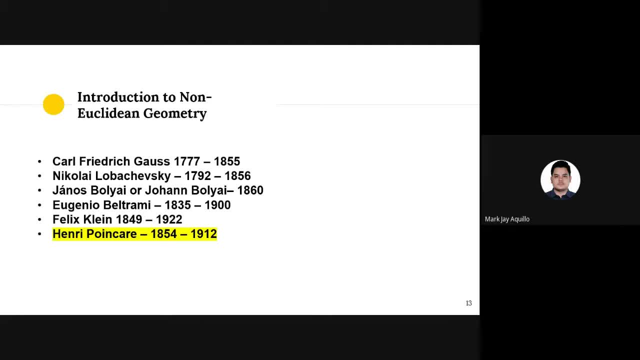 but at least in the spherical geometry we're going to talk about distances of one place to another on a surface of a sphere using only coordinates. we're going to measure distances from one crater to another, distance of a moon, using only the data from NASA on their coordinates. 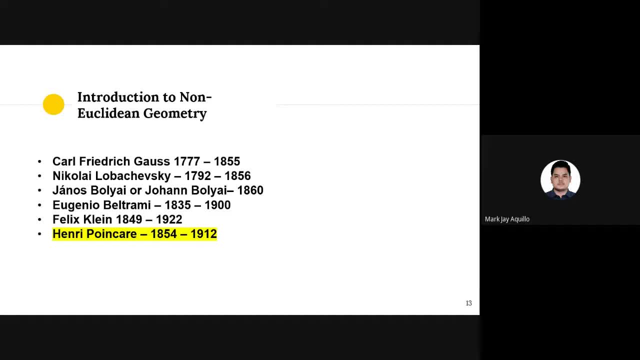 we're going to approximate the distances, let's say, from your place to, let's say, a famous place like the- what famous place is it? like the Mayan volcano, for instance? using only the coordinates from the internet. so it may sound like it's simplistic, but we're going to use 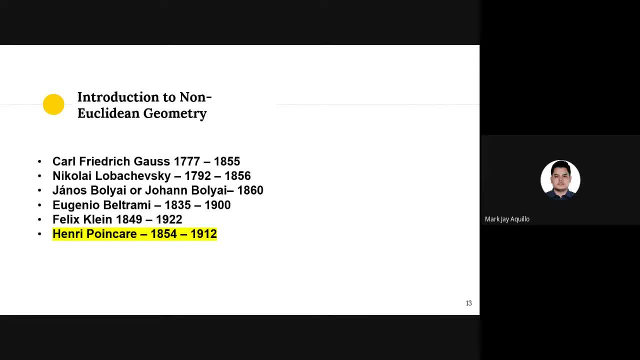 matrices. we're going to use a little bit of calculus in order to finish the computation. although nowadays you can easily use google maps to immediately get the distance, it's always helpful to know the computation behind them, and so on. we will have lots of manipulation on the surface. 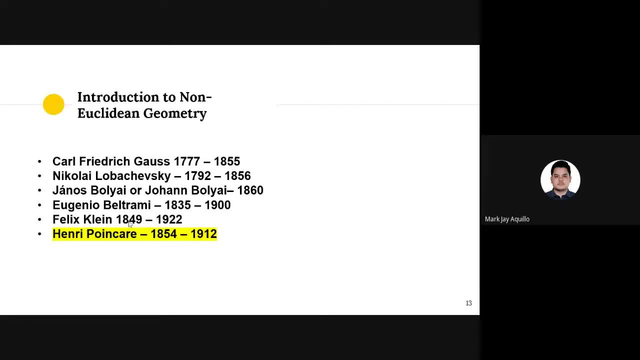 of the sphere, now of the three here. the extension of the spherical geometry was begun by Eugenio Beltrami, and he did it by generalizing the sphere. if you remember your mathematics in high school or your classical geometry, if it was included in your lessons. 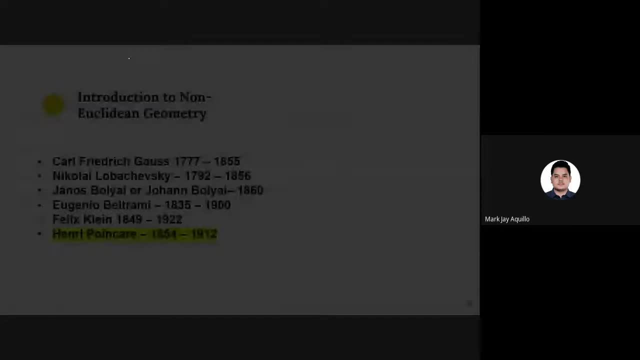 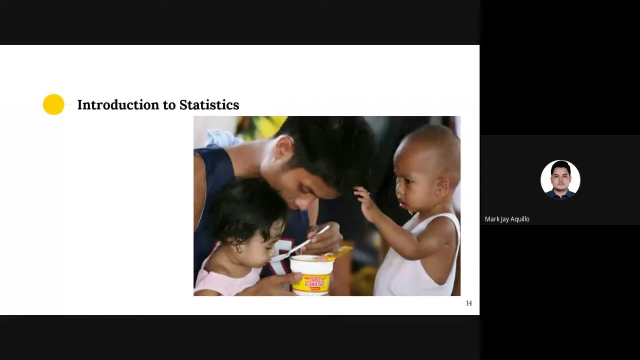 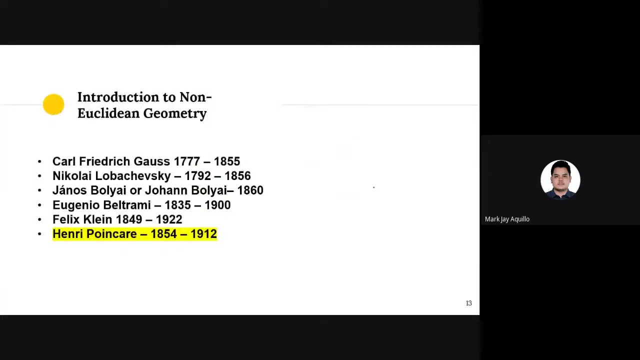 a sphere's equation is sorry, what's the sphere's equation before I write it on the slide? anyone who remembers the equation of the sphere? the unit circle is x squared plus y squared is equal to one, so a sphere could be similar to that to that effect. 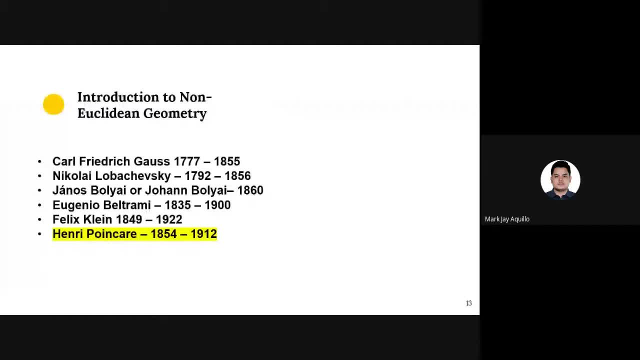 so, for those who can remember the general equation of a sphere, write it in the in-call messages for motivation, plus three participation points. for those who can remember the general equation of a sphere. I'm giving you 60 seconds. while we're waiting for your answers, I'm going to type down: 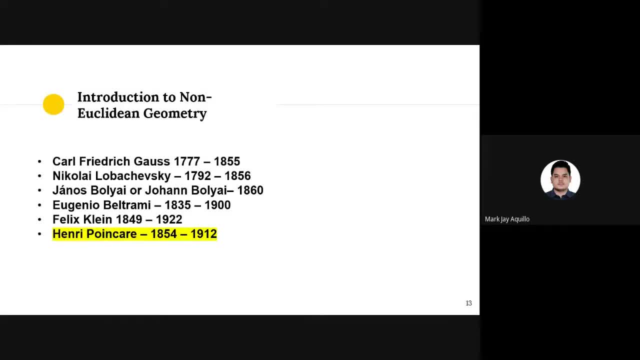 the pronunciation for, so that you would you know, remember it. it's a pronunciation of, that's the name of, or Henry in English, anyone who remembers the general equation of a sphere. no one going once. the general equation of a sphere is sir. yes, friends, you're typing it. 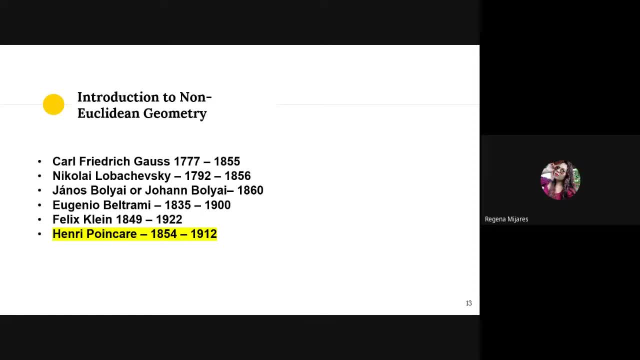 sir. try, sir. okay. yeah, generally that's correct. somehow that's two points though, plus two participation points. Regina, yes, you're raising your hand. yes, sir, x minus a square plus y, my. ah wait, sir. close and open parenthesis. x minus a square plus close and open parenthesis. y minus b square. 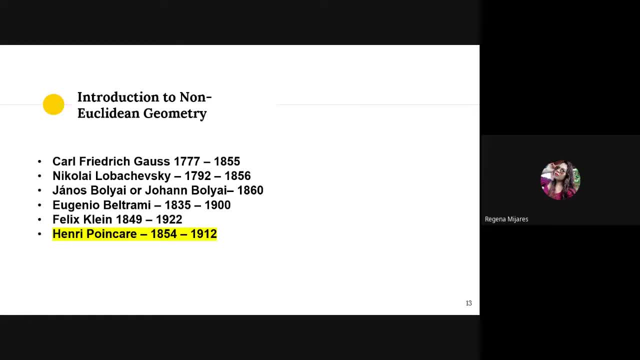 plus z minus c. close and open parenthesis. square. hello sir. yes, thank you, Regina. that's last one. yes, friends, same sir, same as Regina, but I'm. it has different in. that was but big um, the quantity of a minus a squared plus the quantity of y minus b. 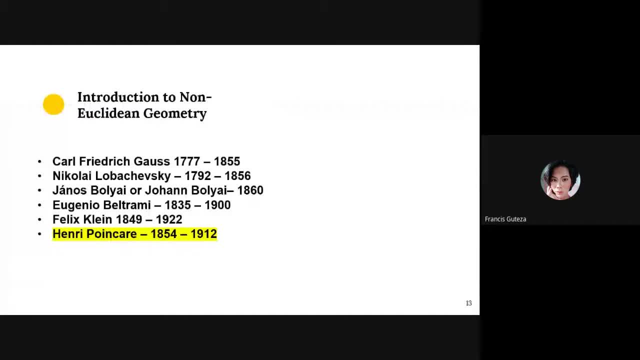 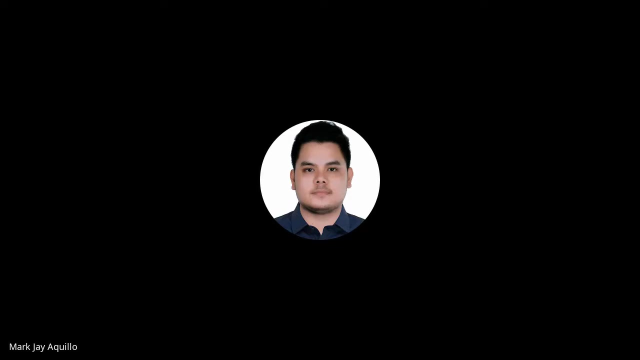 squared, that's the quantity of z minus c squared is equals to r squared. okay, thank you very much, friends. now let's reveal the correct answer for units here: generally: x squared plus y squared plus z squared. now what is he saying? I'm still here, hey, sorry. 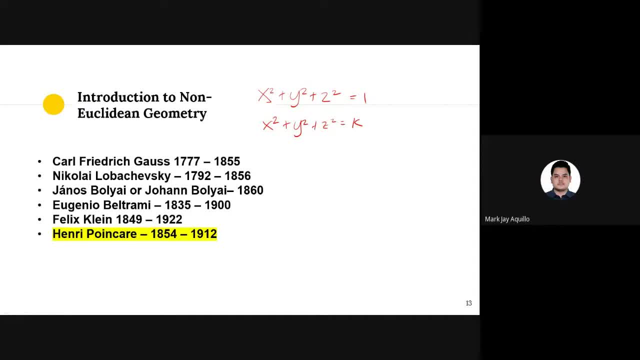 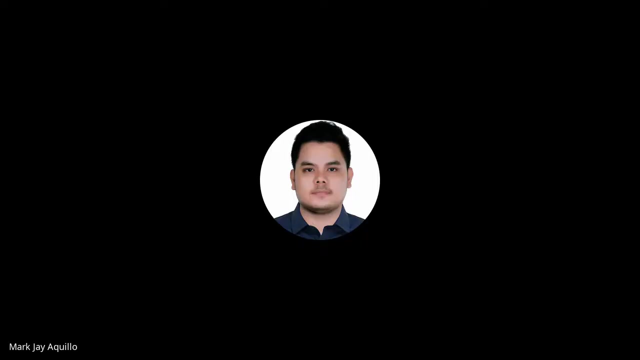 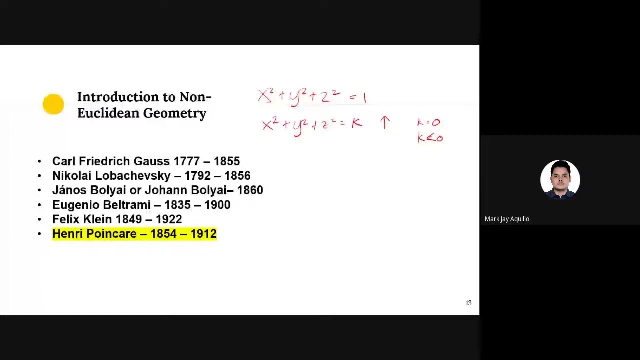 okay, going back, it's x squared plus y squared plus z squared equals k, where k determines the size of the circle. it's basically the radius. the larger the value of the of k, the larger the circle is. the sphere is less than zero. like negative one, negative two, negative three. 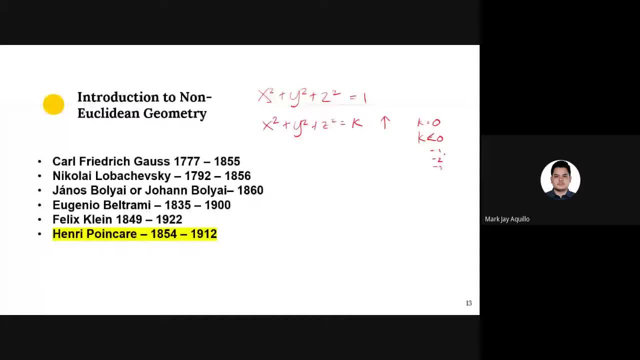 then the sphere cannot exist, because where would it reside, you know? after zero, after nothing. where will it exist? maybe on the other dimension, not in this dimension. we're going to draw the sphere now. going back, Eugenio Beltrami generalized the sphere and he found out: 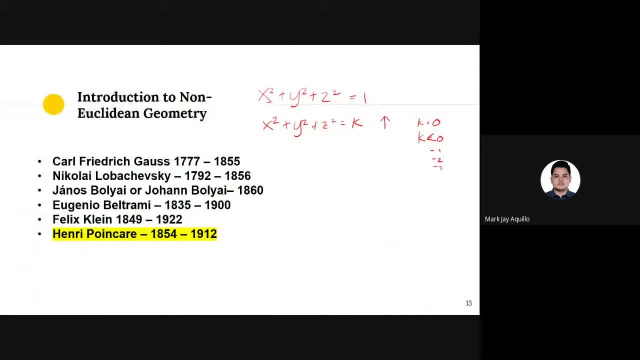 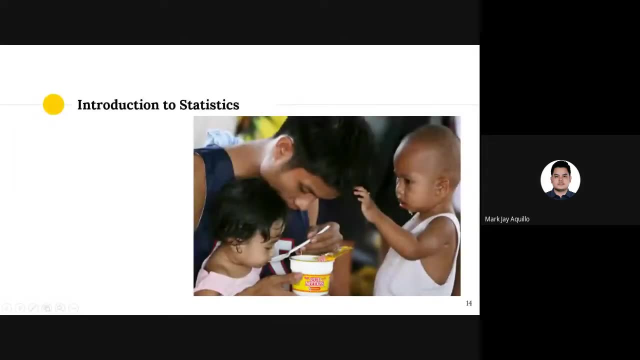 that if he is going to change one thing on the equation, the different type of modern geometry arises now. you have to remember that the first type, the first type of modern geometry that was discovered, was the spherical geometry. so I'm going to write it down here so that you can use it. 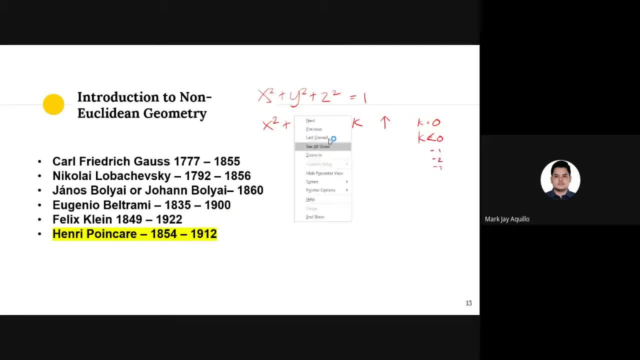 for comparison. so the first: keep going back on that picture of family. so the first one is spherical geometry, where our go investigate what happens on the surface of a sphere, ok, second is, I mean Eugenio Beltrami changed the general equation of the sphere and what he did is only change. 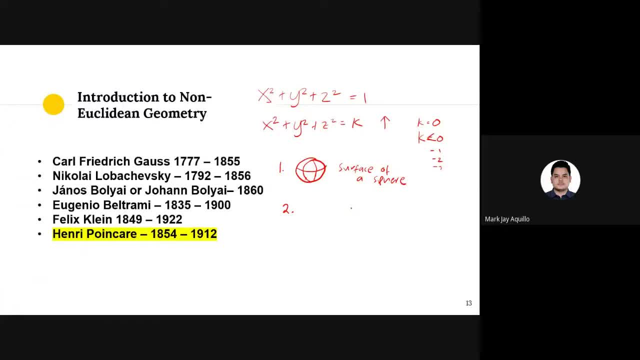 one sign: very simplistic, very small change, but it changed the entirety of the interpretation of the spherical geometry. it became x squared plus y squared minus z squared is equal to k for values. for values, that is equal to zero. if k is equal to zero, I don't know. 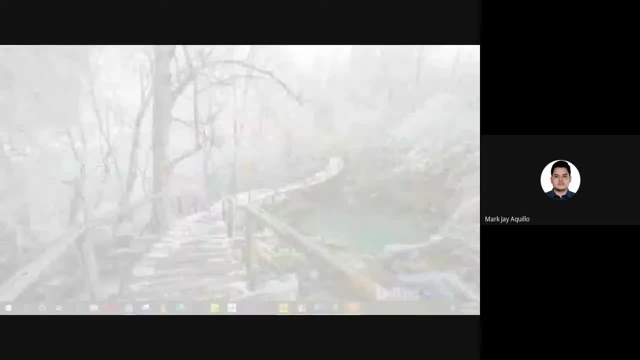 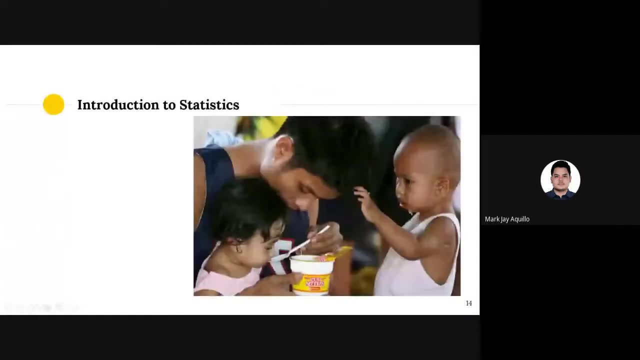 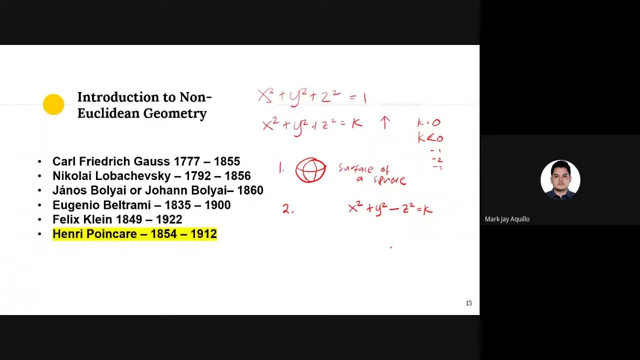 what's happening? it keeps on going back here. this guy wants to be seen. ok, so if it's k is equal to zero, what we form is, if we're going to draw the xyz plane is a cone, a cone here. so this cone is the result of. 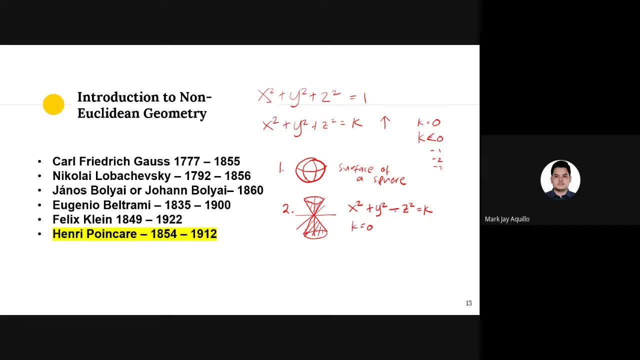 reversing the sign on the z and the modern geometry involving the cone is a geometry involving the surface of the cone. now we can draw triangles on the surface of the cone. we can draw lines on the surface of a cone. each of these things have their own interpretation. 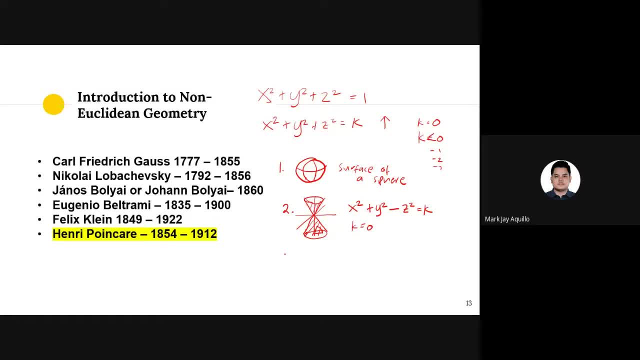 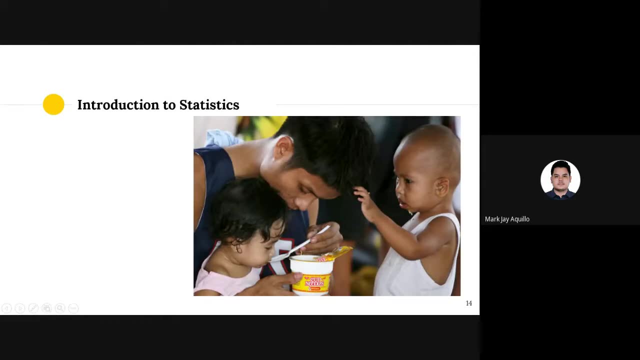 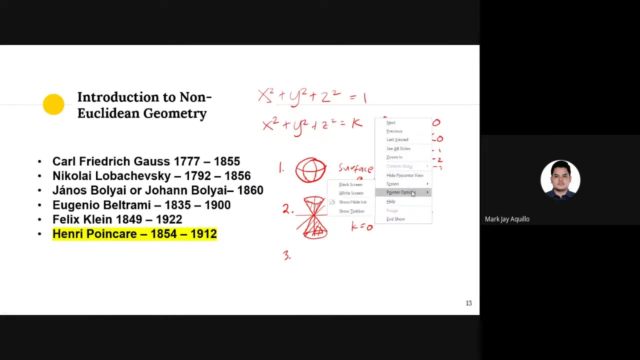 when it happens on the surface of a cone. the third type of geometry is when k is equal to one, and when k is equal to one it forms a different type of geometry, called a hyperboloid. I need to take note of this because I don't know. 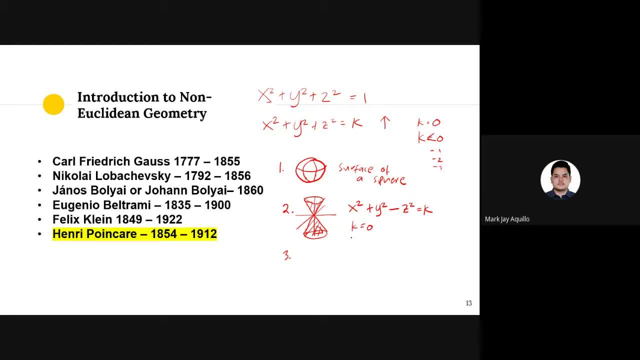 maybe I'm going to lose it, or maybe because it's not part of this slide, this one is conic, just okay. now hyperboloid is like this: it's like a tube. so that's hyperboloid. and the fourth one is now. hyperboloid happens when 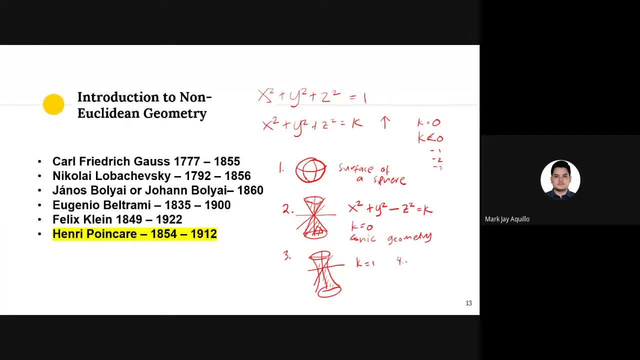 k is equal to one. now, when k is equal to negative one, what happens is we have a hyperbolic plane. so this one is a plane. this one is a plane too, and they're not touching each other. this plane has finite size, but the surface goes. 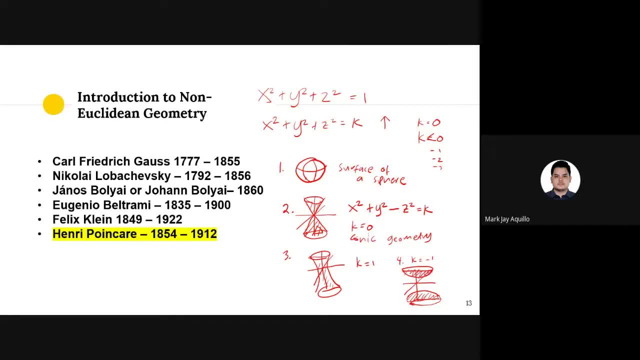 infinitely, like: from here you can go to the side, you can only approach the side, but you can never touch it. okay, so I'm going to show you, I'm going to stop my presentation here, and then I'm going to show you the different geometries when they're rendered. 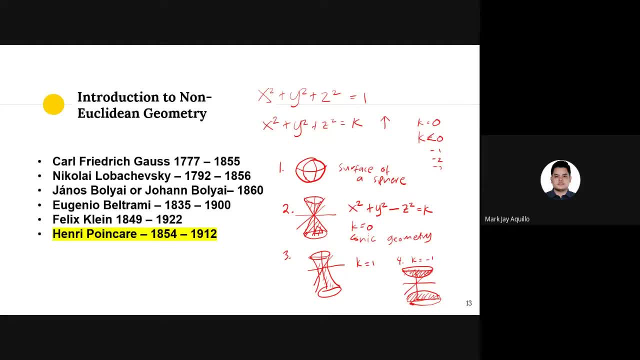 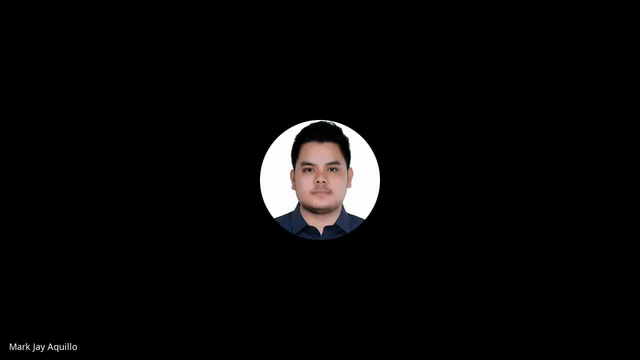 using computer whiteboard so that we can write on the. you know, on the surface we're about 10 hour lesson, though so far. can I get your opinion on modern geometry? it's something that you might have liked, or does it sound boring? what's your opinion on that? 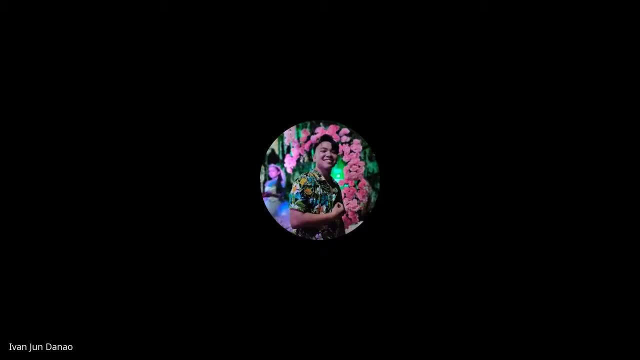 they're good in history history, yeah, the history of mathematicians. I enjoyed it too. yeah, history is only like introduction. okay, guys, but the topic, sir, I'm going to talk about, history. okay, maybe you need to consider changing major what? so the first one that we're going to talk about, 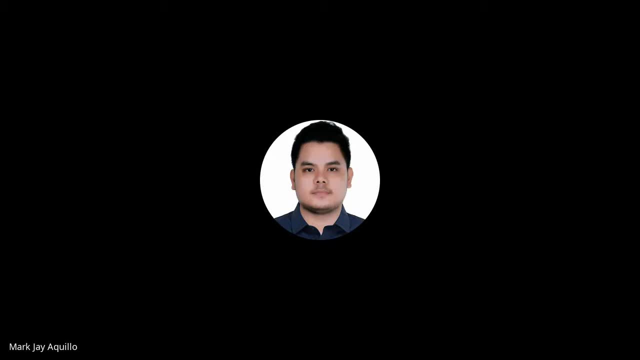 I mean we're going to see is a sphere. I'm going to show you a sphere so that we could try to check whether we could draw a triangle on its surface or not. only problem is here, so it's black. I hope you can see your screen now. 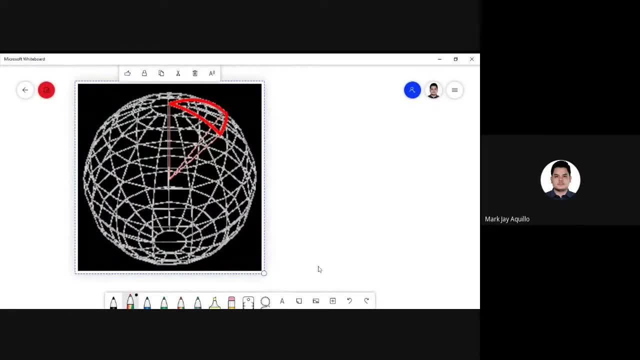 although the picture that we have is black. can you see it? can you verify? now, look at this: on the surface of the sphere, you can draw a triangle, and that triangle will have- this will have- properties too. just like you know, just like a regular one moment I'm trying to exit. 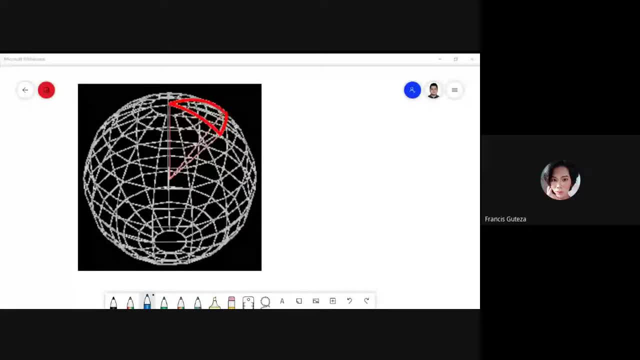 a window. hello, sir, yes, let me clarify. okay, sure, those students who give you the formula of the sphere by this participation. yes, yes, okay, sure, okay, that's very good. now let's have friends. yes, sir, okay, thank you very much. friends, let's have an overview of. 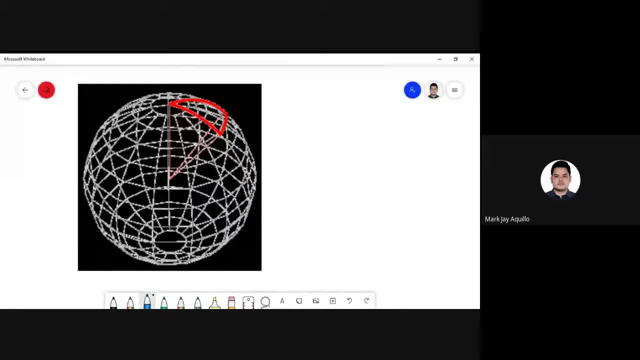 geometry of the sphere. look at this: similar to the regular, the uniform plane. we can draw a triangle here, and a triangle could have angles as well. take this one. you can also draw a point you know at the if you're going to look at the globe on top of the globe. 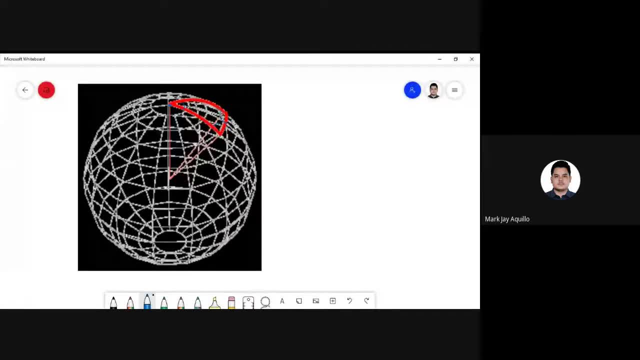 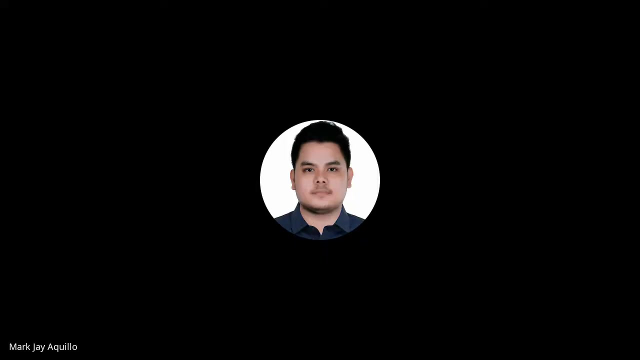 on the north pole, there's a point at the bottom of the globe. there's also a point. you would notice that all of the longitudes would connect the point on the north pole and on the south pole. you can see that the, the, the, the, the, the. 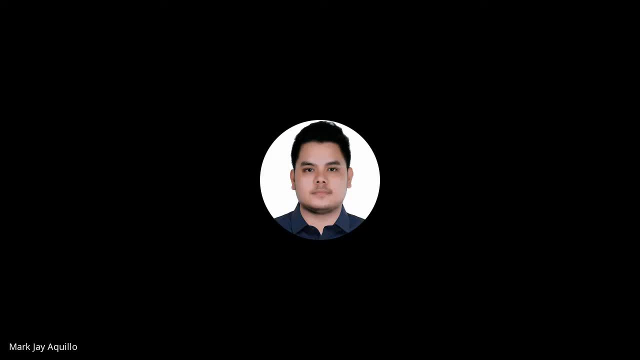 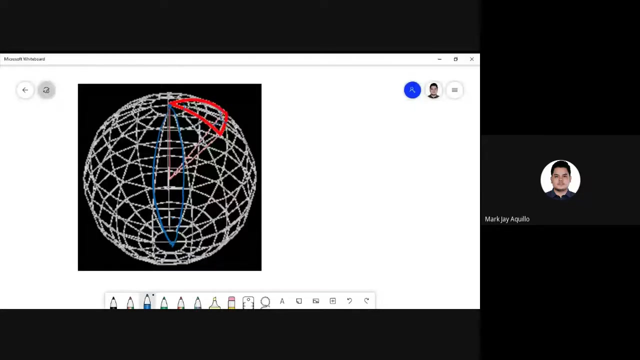 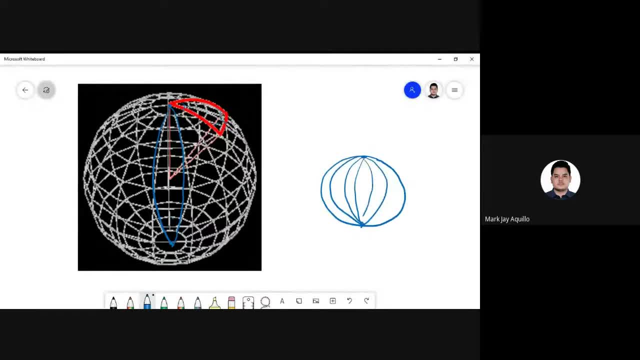 number of geodesics can be drawn to demonstrate that there's an infinite number of lines that can be drawn connecting two points, And that is in the surface of a sphere. Also, in the surface of the sphere, you will have this type of figure And also have you know a different formula for. 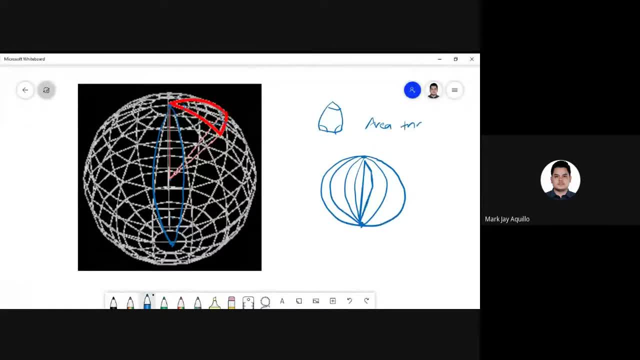 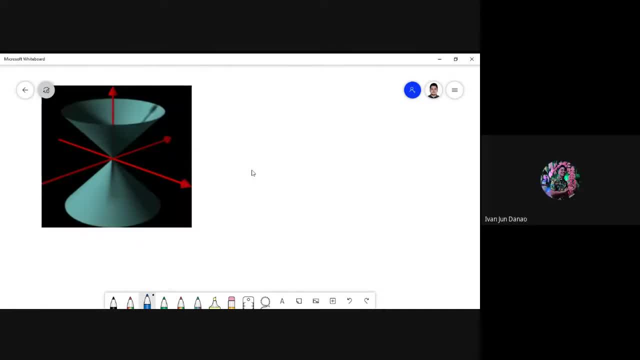 generalized geometry was formed And I'm going to show you the conic geometry formed when the generalized. but to be very honest, I'm not familiar with conic modern geometry. this is a very high, higher mathematics, so let's proceed with hyperboloid. hyperboloid. 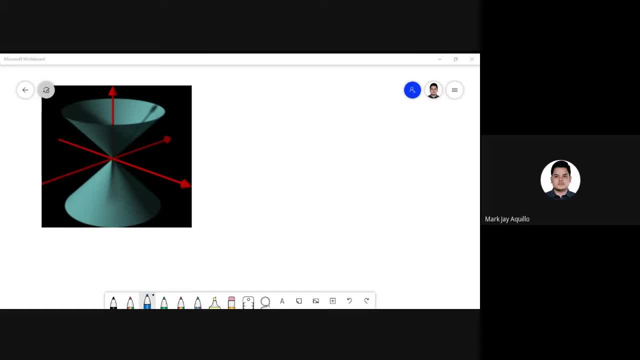 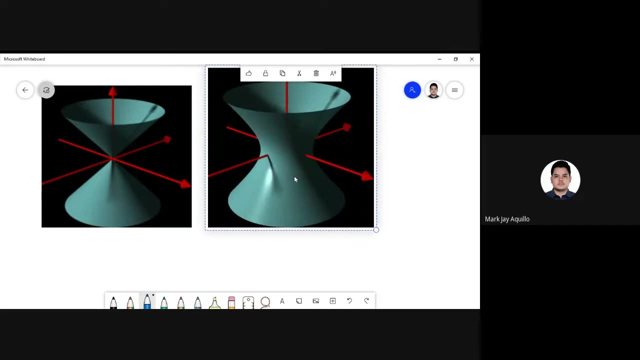 happens? at what value? again, one is equal to one. why? this is what a hyperboloid looks like. can you identify a real-life object that closely resembles a hyperboloid? do you have something in mind? yeah, a funnel that more symbols. a cone right chinese yo-yo. 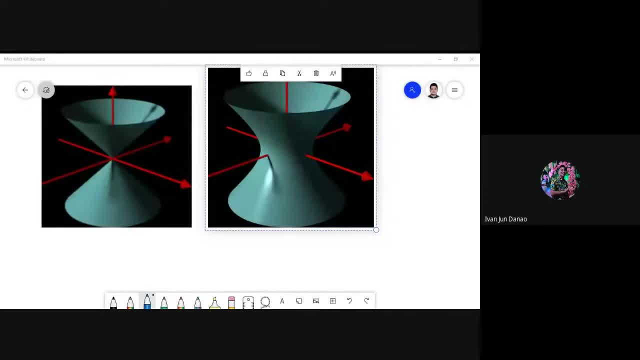 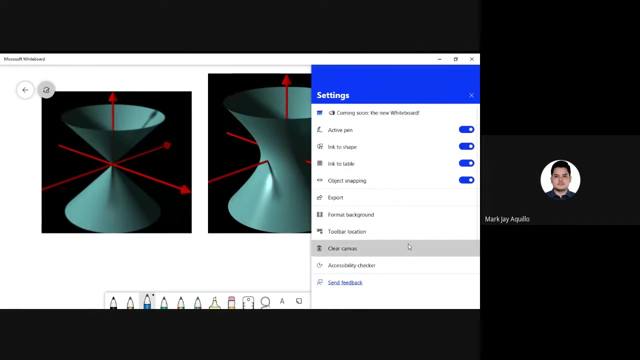 chinese? what chinese yo-yo? yeah, yeah, somehow, sir. plantation, plantation, plantation. yeah, it looks like it. how about the exhaust of a nuclear power plant? looks like hyperboloid as well. I think the third one that I'm going to show you, the hyperbolic, for me, is the most interesting. I don't know, I don't know about other mathematicians or other- 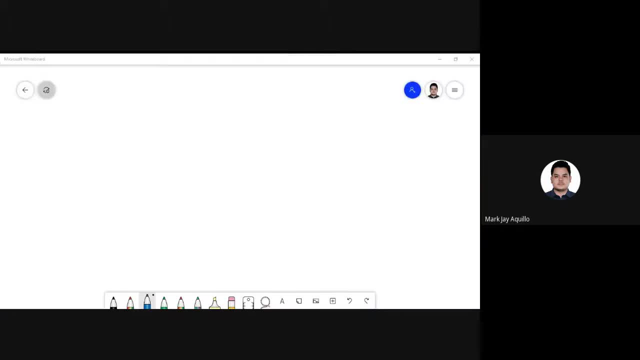 mathematics teachers, but for me the hyperbolic plane is the most interesting of the three. the reason for that is one moment I'm going to show you. I'm going to show you only the bottom part of the hyperbolic plane. you can, you know, this is the bottom part of the hyperbolic plane. 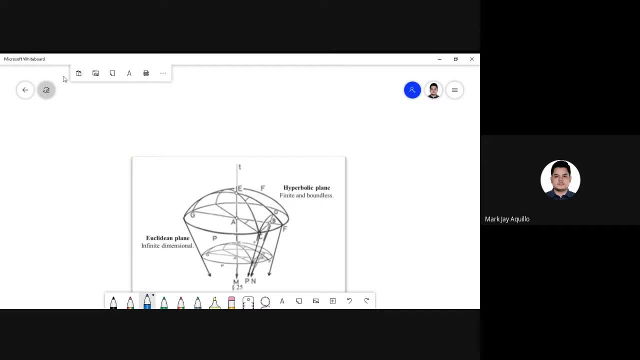 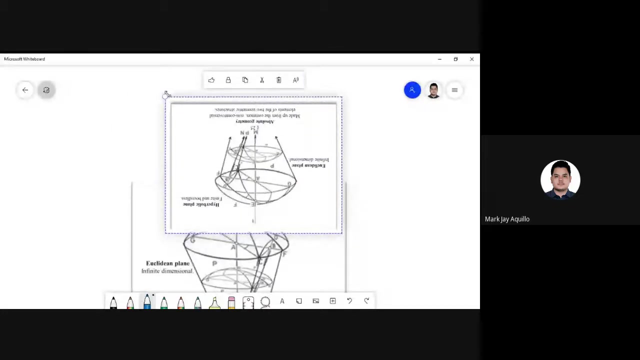 if we're going to add the upper part, all we need to do is just to flip this like this and we'll have the upper part. so yeah, that's the upper and the lower part of a hyperbolic plane, just to demonstrate that there are two parts: the upper and the lower portion. I'm going to remove the lower part because I don't want to lose the upper part of the hyperbolic plane. so we haven't managed to eliminate either from the upper part. I'm going to build the higher part there and I'm going to put back this leg in front of the upper part. so here, just one 저녁. 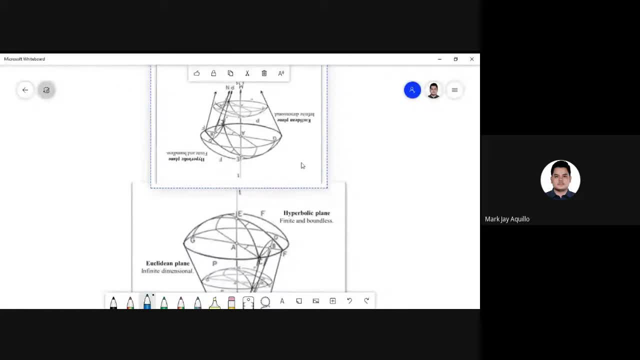 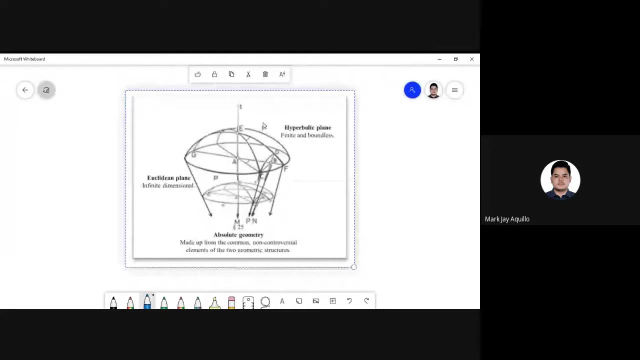 I'm going to remove the upper part so that we can focus on one hyperbolic plane at the same time. So a hyperbolic plane for me looks like a convex lens. I'm going to emphasize that a hyperbolic plane begins and ends here. 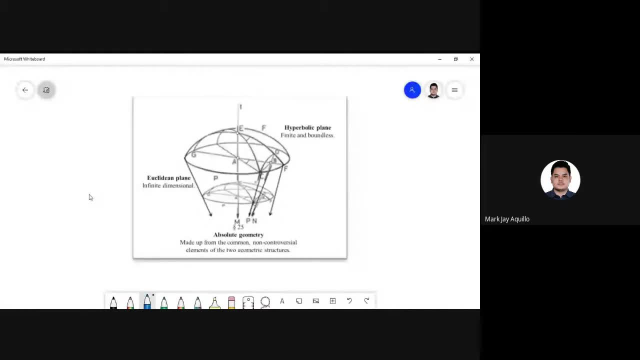 So the hyperbolic plane is basically here. Sorry for the excess line. This is how I could draw in the image. The hyperbolic plane is mostly just this. This is the hyperbolic plane. It looks like a convex lens. 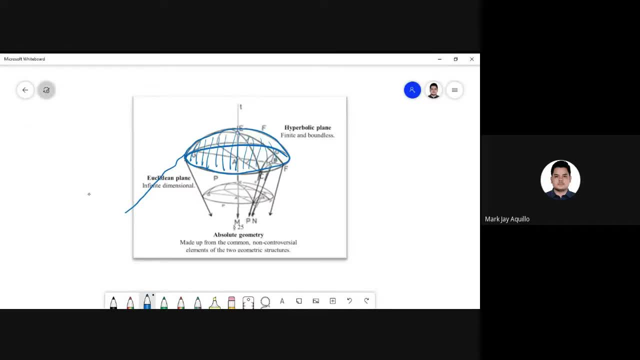 Now, what's interesting in this type of plane? what interests me about it is the fact that you can move from the center here to here. You can travel indefinitely, but you're never going to touch the end. I don't know what happened while there's a triangle here. 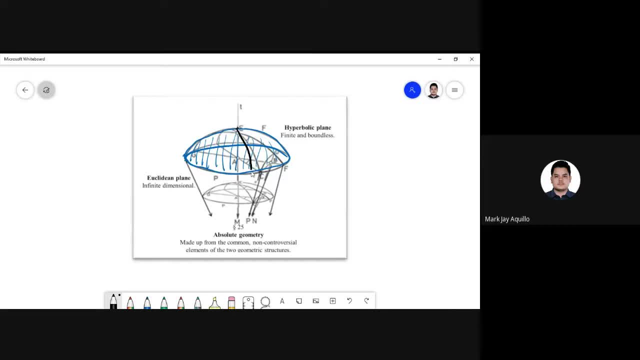 So you could travel to the end, But- But on this edge, you can never touch it. This edge is basically like an asymptote, where you can only approach but you can never touch. So what happens if you look from the top? 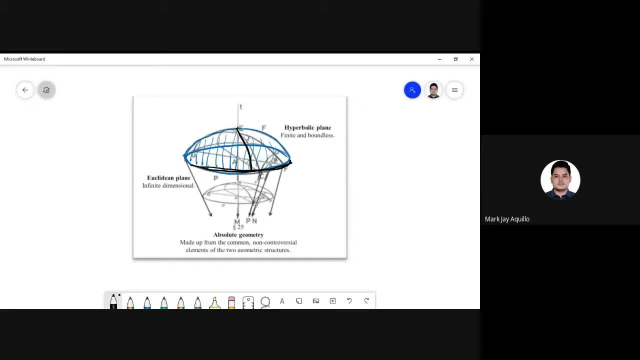 and you will have images drawn on its surface. I'm going to show you a famous artwork using the hyperbolic plane. This was the cover of the book of Philip Zimbardo in his book called The Lucifer Effect, But I can't find the exact image. 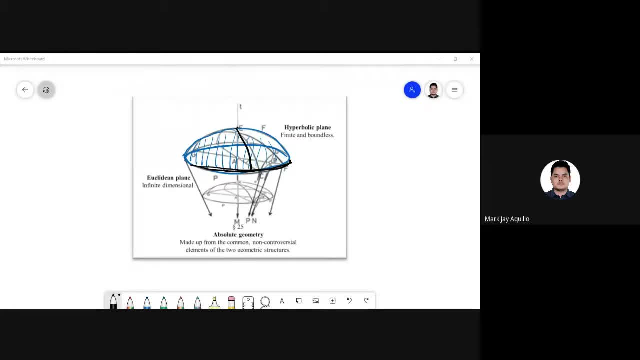 So here, So I'm going to show you an example of an artwork, I mean of a hyperbolic plane from above. This is an example of a hyperbolic plane from above. This is an artwork, It's like an optical illusion. 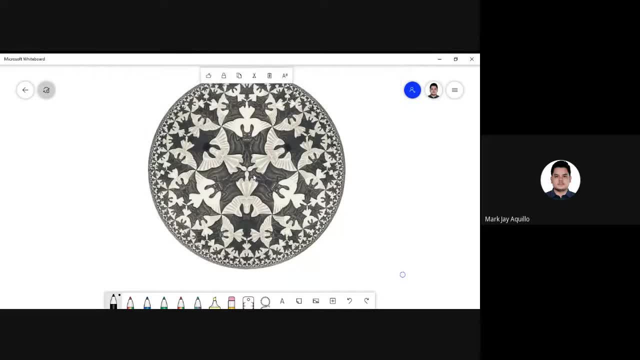 If you look at the black part, you will see the devil. If you look at the white part, you will see angels And you would notice. Okay, I'm going to ask you: What do you notice about the pictures as? 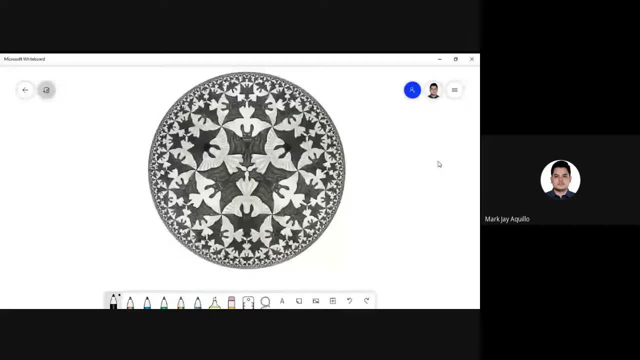 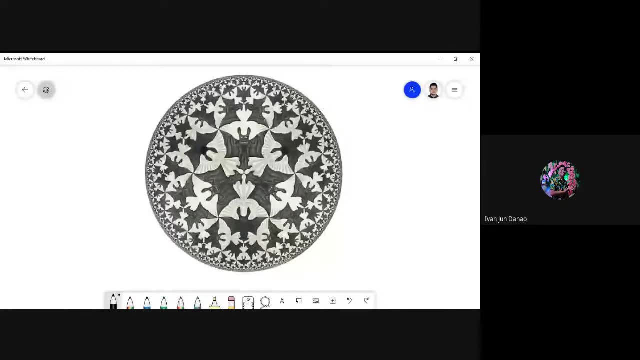 they get nearer and nearer to the edge of the hyperbolic plane. Anyone, What do they look like, sir? From the top, They are small sir. What do they have? Was that you? What did you say? Bigger material. 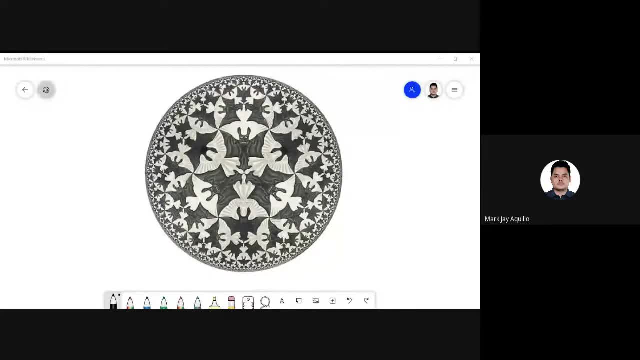 What do you notice, Regina? The pictures. What do you notice about their size? As the pictures move towards the edge, The picture becomes smaller. They become smaller, sir. They become smaller, But Yeah, But they don't approach the edge. 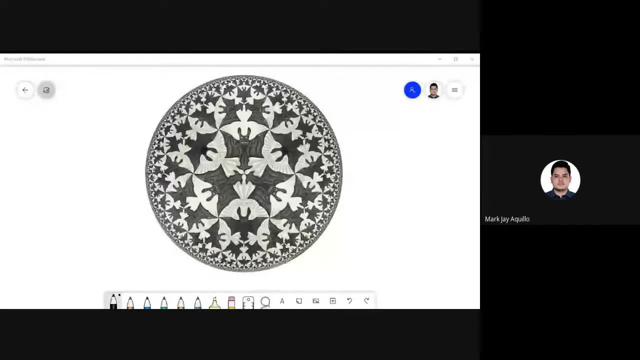 That is the most interesting aspect of a hyperbolic plane. Now you're wondering: What are the implications of this modern geometry? Why do we need to learn modern geometry? Remember the story about Newton. We're about to end our lesson. 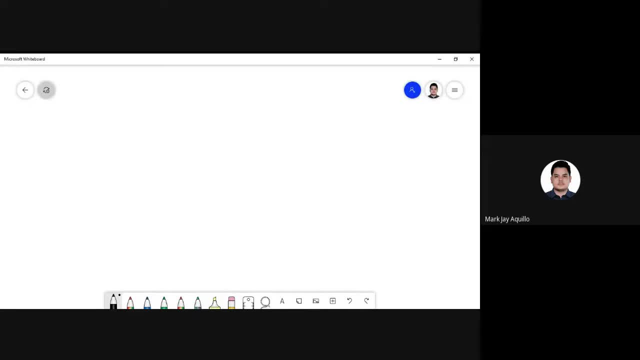 And this is our end story. Remember the story of Newton? Newton was supposed to. The story goes that he sat at the bottom of an apple tree And an apple fell before his eyes. And then he realized the apple fell. 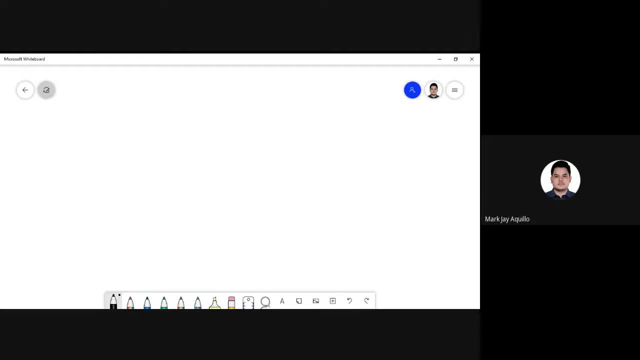 because of the action of the force of gravity. From then he was able to generalize the movement of objects in the universe using the concept of gravity as a force, And he said that the pulling force of a gravity is directly proportional. 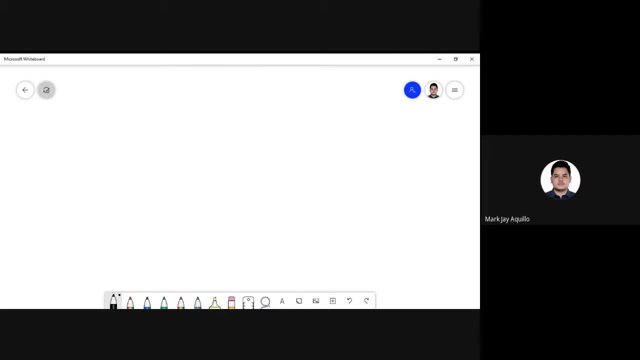 to the distance of an object being pulled to the center of the object, In this case a planet. Now, years later, Albert Einstein came with two most important works. We call them now the general theory of relativity. 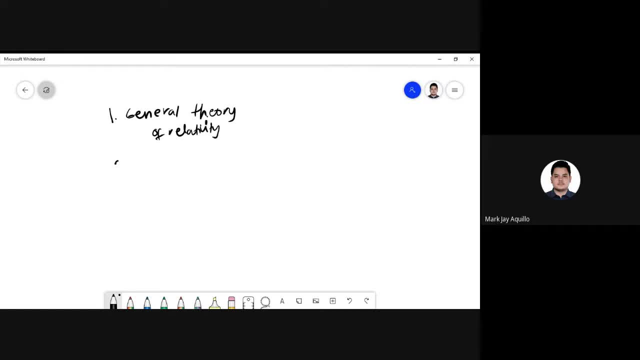 and the special theory of gravity, And, according to Einstein, gravity is not a force, Gravity is a consequence. Imagine if we have a plane as a space, If our space is plain Like this one. 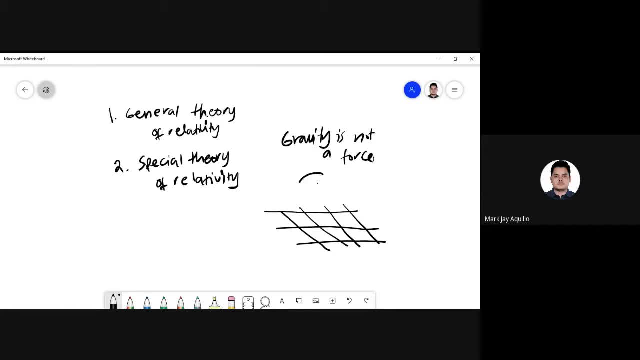 And uniform And you put a very heavy object on top of it, Then the plane is going to curve This one To accommodate the mass of an object. Now you need to remember I'm not very good in drawing. 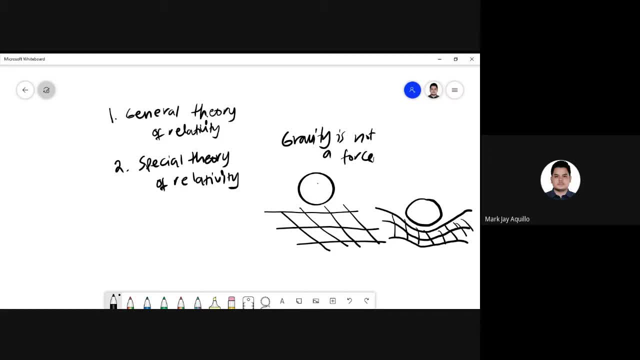 And you need to remember that when we say space, we're actually referring to a grid of space and time, Or space-time, And, according to Einstein, very heavy objects like the sun and the earth curve space and time. 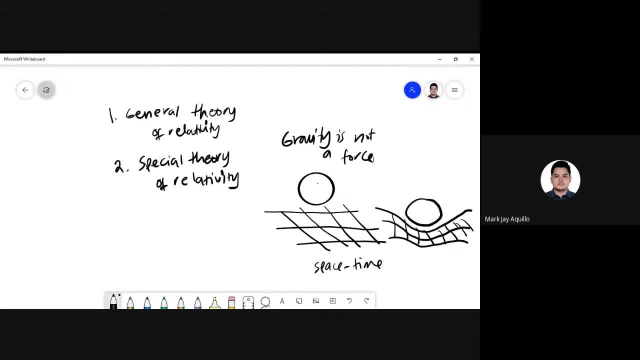 And this curvature around them makes all of the objects fall. I'm going to show you an example. I don't have an example for that, But what happens is, instead of the sun, pulling the earth close to itself. 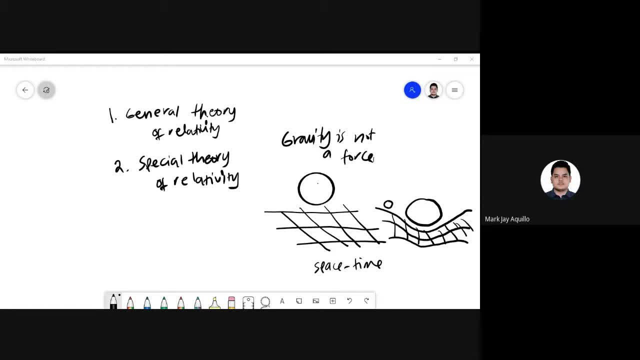 or the earth pulling on you. the curvature of the space around the sun allows the earth to fall into it, And the curvature of the space around the earth allows us to fall into it, creating a gravity. well, We're falling. 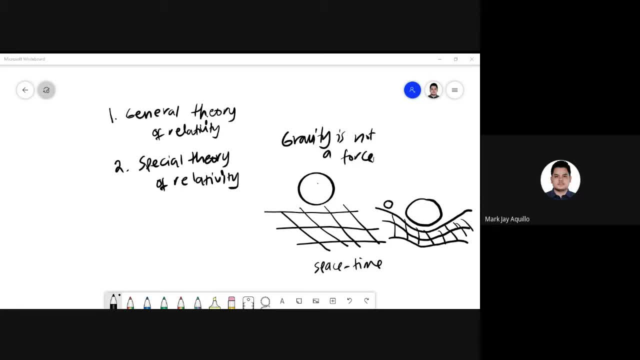 because of the curvature of the space-time And if you watch the movie on Interstellar, It was demonstrated there very well. Interstellar revolved around space travel And there's a scene there where they worked on a spaceship. 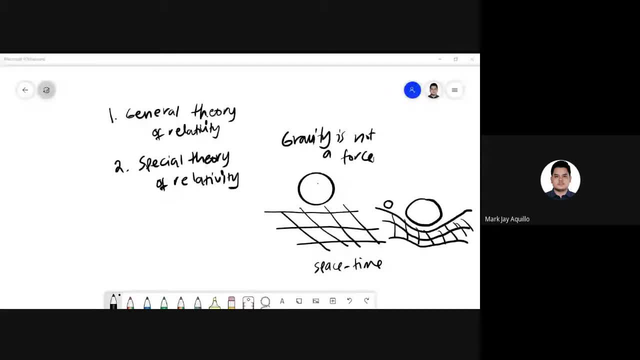 near a black hole. Remember, a black hole is so massive that its gravity is so strong that no light can escape it. So if it's so massive, then the curvature of the space around it is so steep as well, You notice. 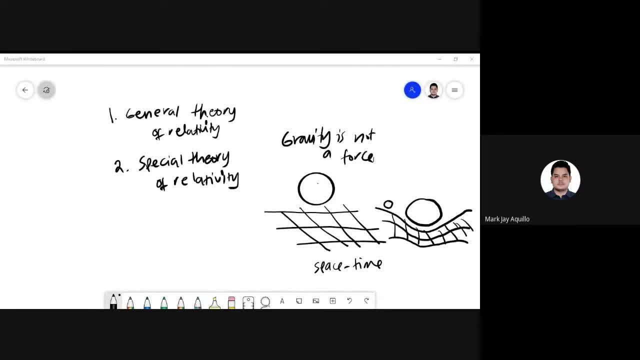 while everybody was getting old. the person on that spaceship was young, Right? So it also influences time. Near very heavy objects, time slows down. Not just gravity becomes very strong, but time also slows down. So this type of physics 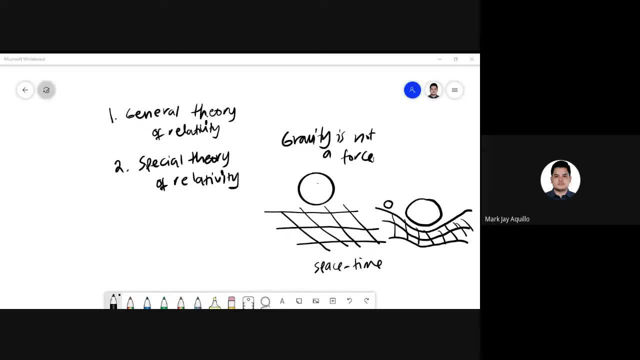 this type of theory of Einstein. the only mathematics that could support it is mathematics on the curved surface, And that is the primary use of modern geometry. Now, if you're planning to be an astronaut in the future or a scientist, 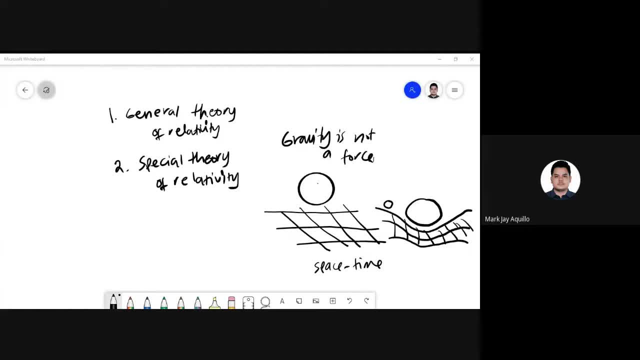 or if you believe that in the future. this type of knowledge is so common because we're so advanced and you want to participate in that kind of future, I think modern geometry is for you. You need to learn that there. 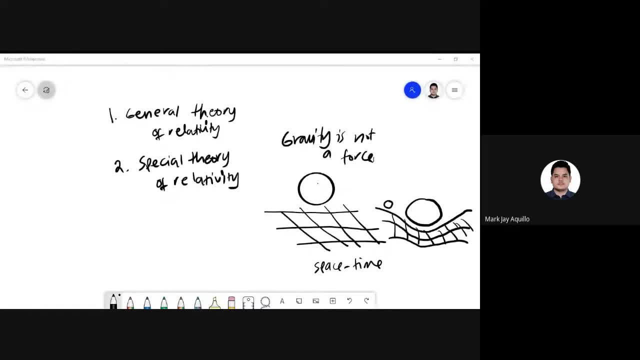 that the space is not always uniform, That there's a region in the space that is either positively or negatively curved, And that, in order for you to have an accurate measurement on those spaces, you need to use a very precise 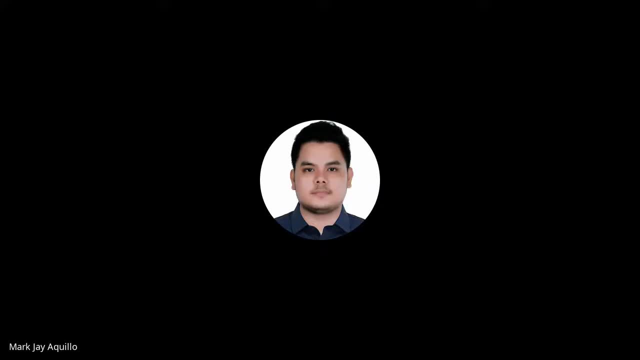 measurement of the area, And that's why we're so interested in the idea of the universe, And that's why we're so interested in the universe And that's why we're so interested in. 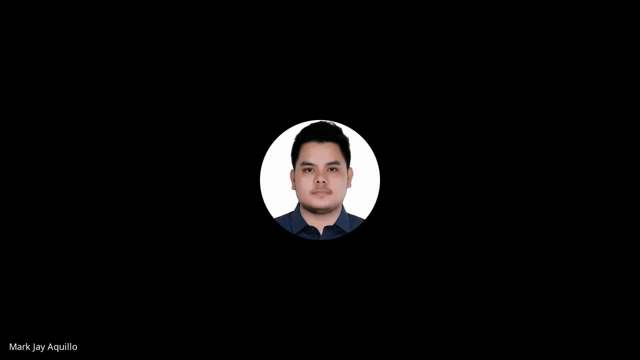 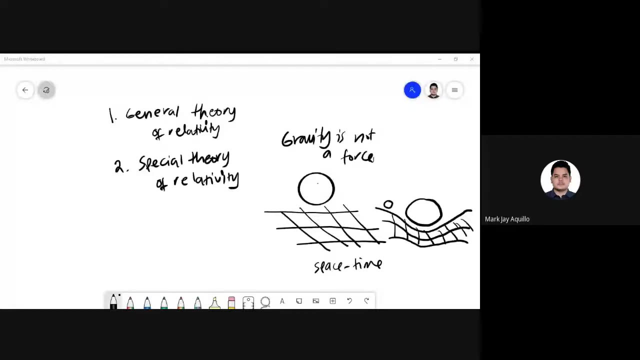 the universe And that's why we're so interested in the universe. Hello, so going back. so again. that ends our discussion on the introduction on modern geometry. In this class, we're mostly going to focus on spherical geometry. 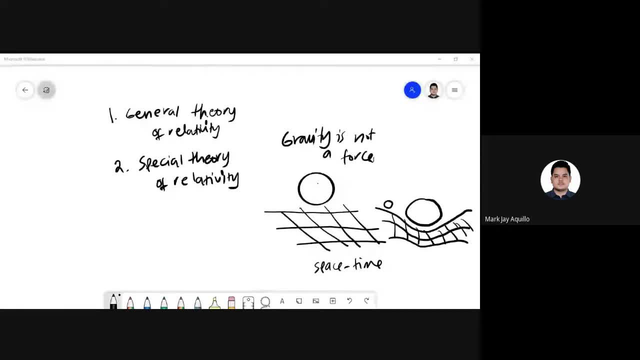 We're going to familiarize ourselves with the formulas involved, with how to compute for the internal angle of a triangle, with how to compute for the area of a triangle. We're also going to talk about the vector, the direction of the forces. 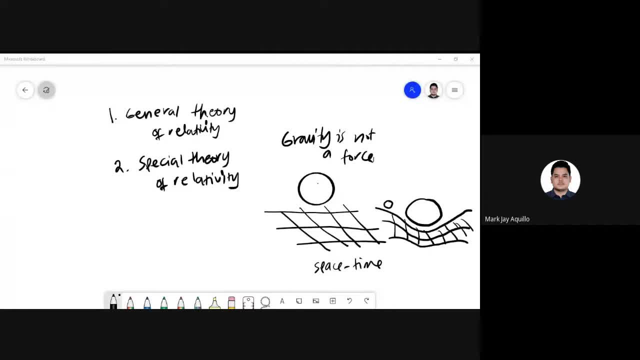 We're going to talk about matrices And then we're going to proceed with computations on the surface of the geometry. Yes, Regina, we're almost done. Now, before we end, I'm going to entertain your questions. Is there any question? 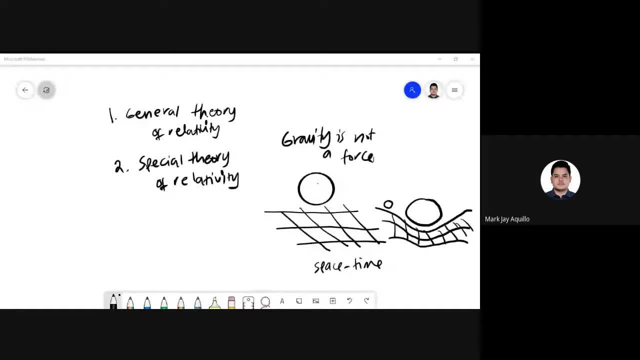 I hope you took some notes because after this, either this evening or on Saturday in the weekend, I'm going to post a quiz regarding the history of the modern geometry. I hope you took some notes. I hope you took some screenshots. I'm going to post the recording of this on YouTube. 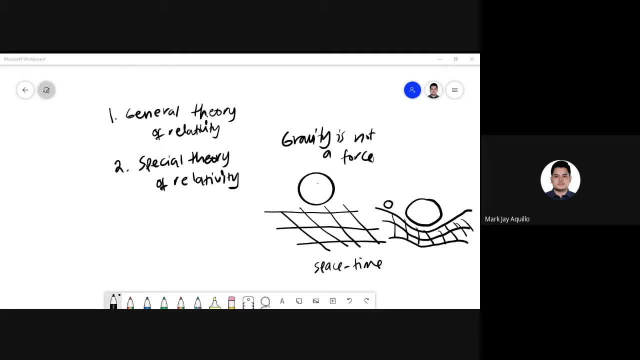 So watch out for it on my YouTube. I hope you review the video because ideally, this is one of you know. since this is introduction, it will be a simple quiz and I hope you've perfected We're going to have a quiz. 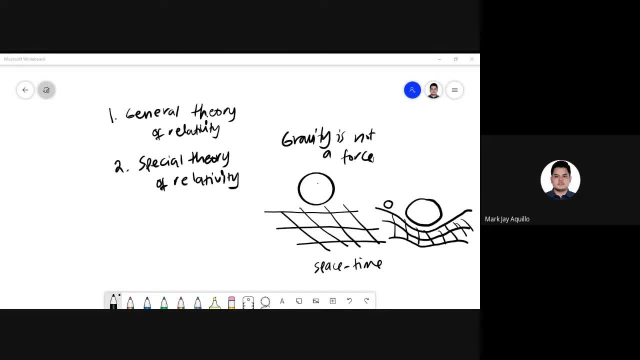 Any question, though, Christine? yes, thank you. Okay, so would you like to you know what The reason I punch? The reason I punch is because I want to encourage you. I always believe that in a certain crowd like your class, 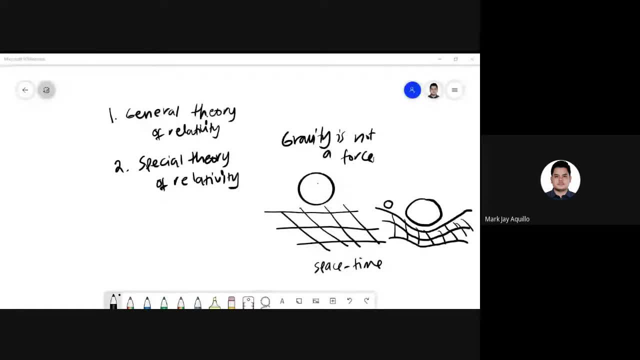 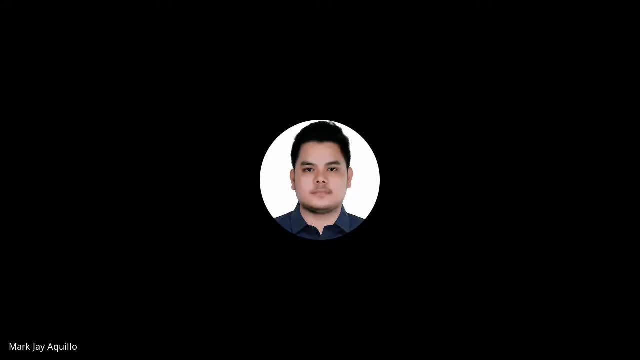 there are some students who have the potential in the future to discover existing mathematics or computer science. So I want to encourage you to do that. I want to encourage you to do that, I want to encourage you to do that. Contradicts and existing mathematics altogether. 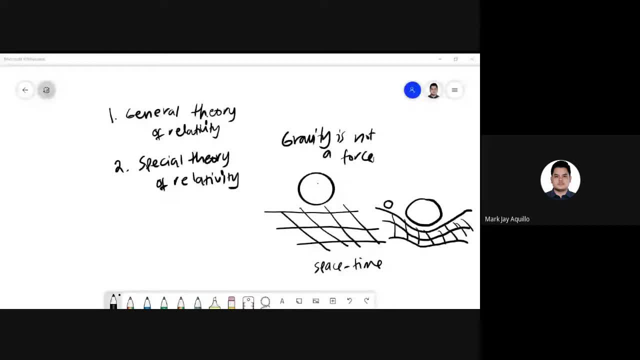 One that is a key player, a game changer. You know, try to explore, try to ask, observe your universe, your surroundings, Ask questions, questions that mathematics could generalize. Ask yourself: is there a mathematics that exists that could help me compute for this? 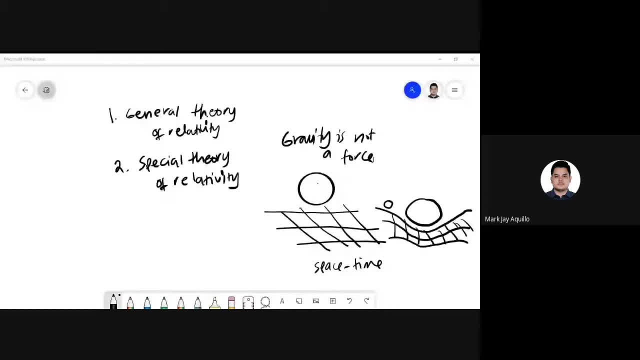 If there is none, maybe it's time that you develop it, And if not, it's time that you create it you. then it will be a proud moment for the best of scott that one of its products has amounted to becoming a mathematician that could go down to history, since there is no question. thank you for. 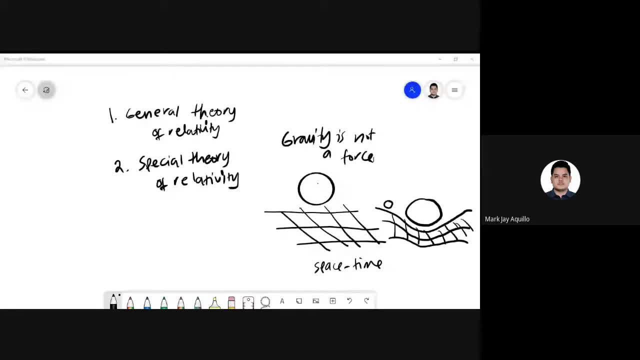 listening to the discussion. friends, please post the names of participants in the google class. yes, sir, others may verify. let's not take pictures of the chat. open your camera so that we can have. thank you, friends. please open your camera so that we can take a picture, hi a spoof, of your attendance. hi, sir haggard. now, oh, christina. 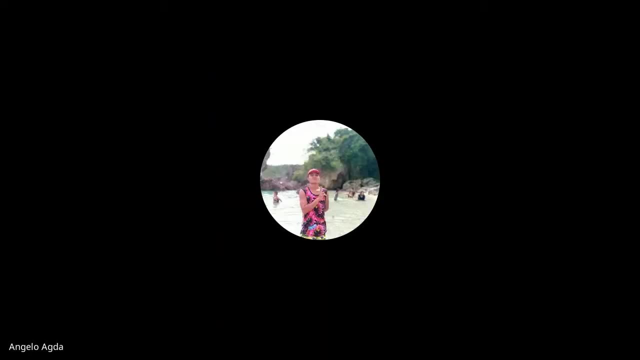 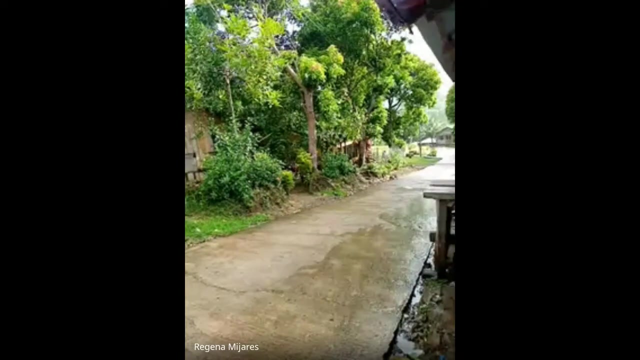 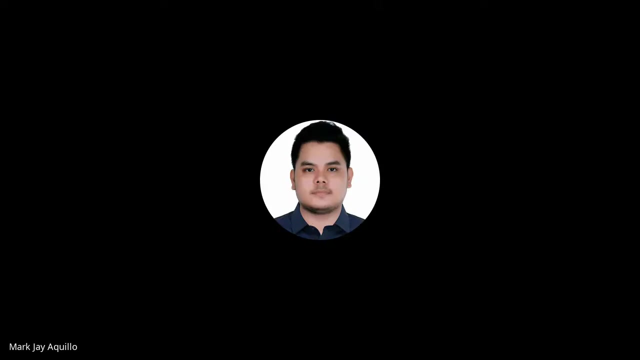 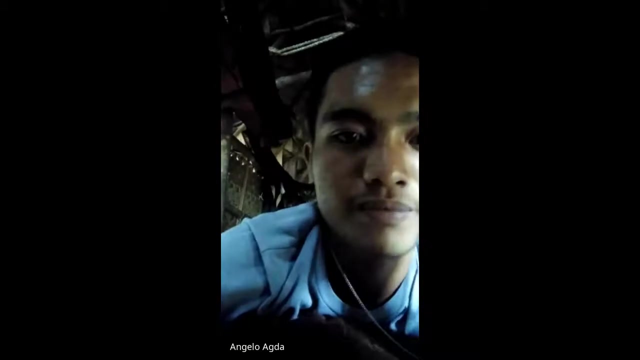 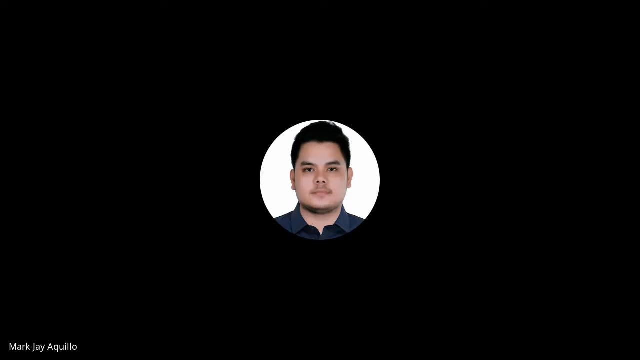 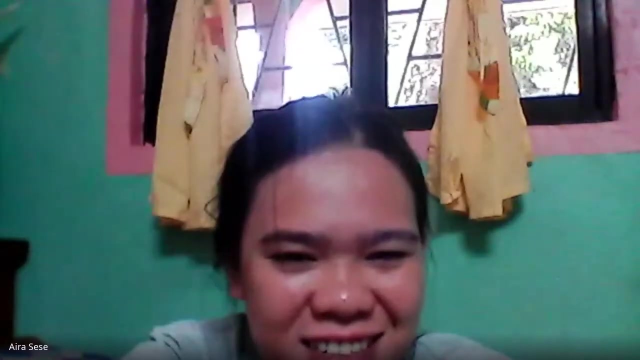 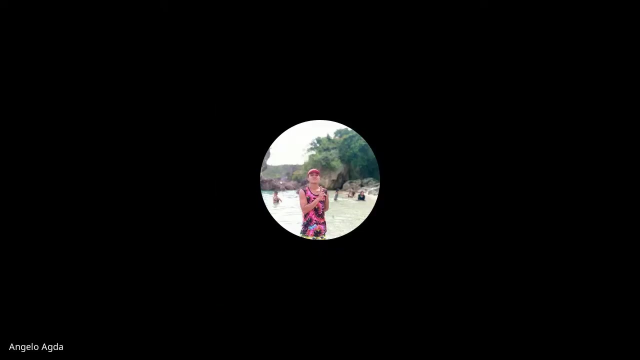 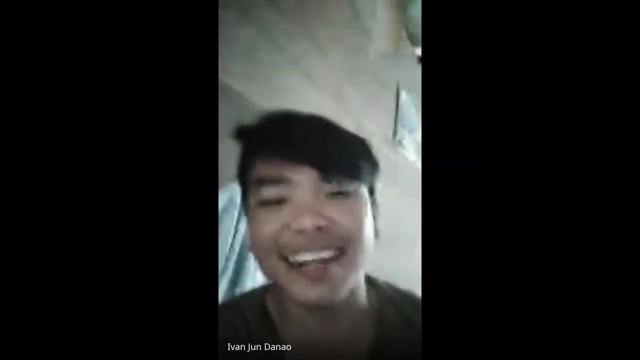 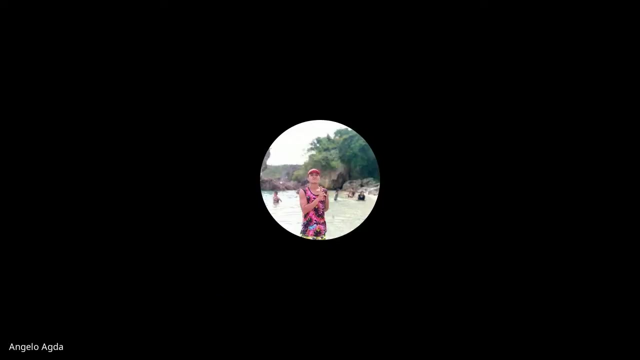 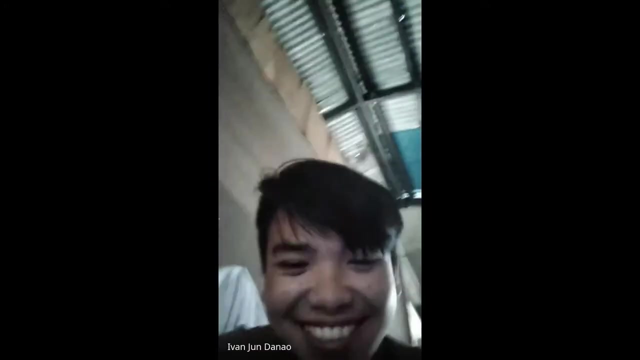 wow, as an accident, excuse me, sir. yes, you're excused. open, come open, come. come on, sir, a moment to encourage others to you know: join, you look beautiful, congratulations, you look like a. oh my god, i will say to you, and this class is a business, thank you, see you next week. 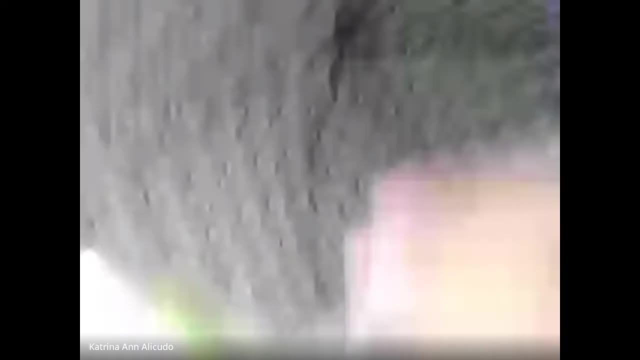 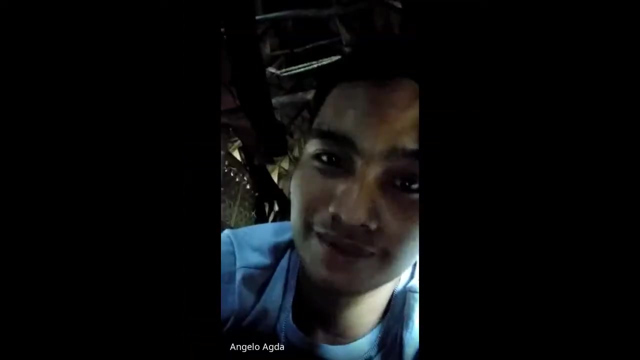 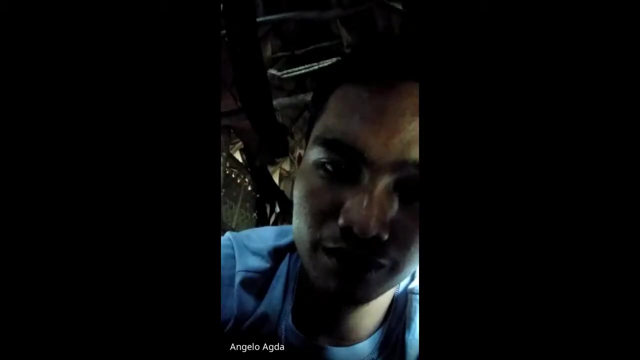 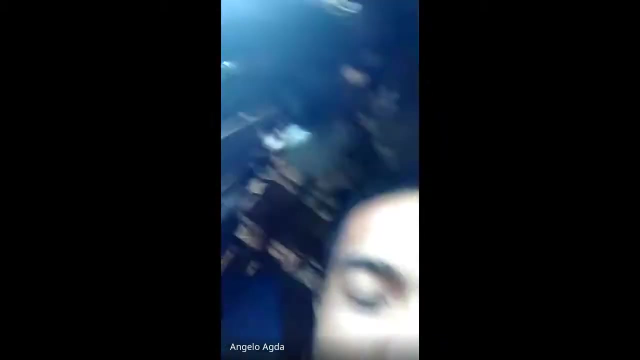 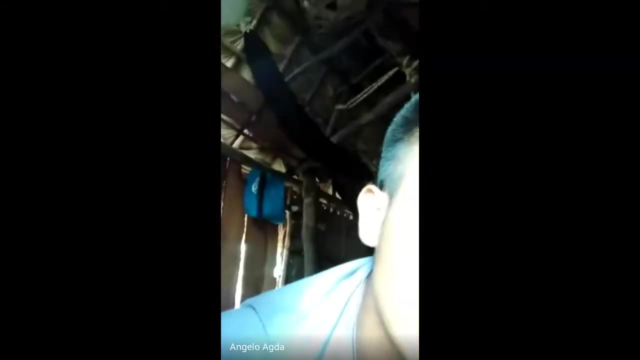 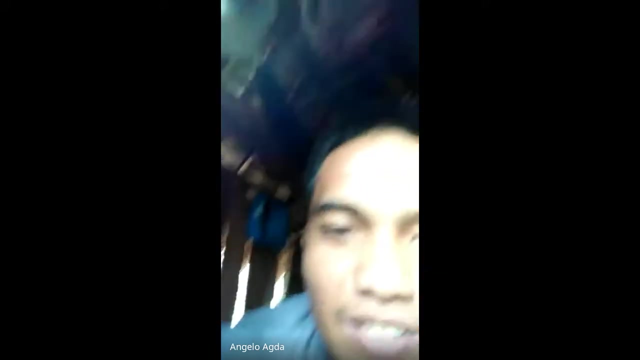 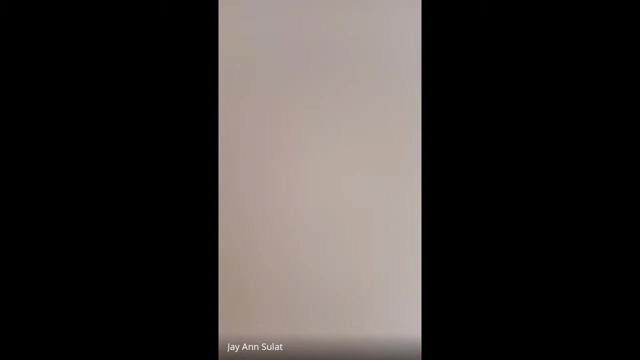 yeah, foreign, foreign, foreign, foreign, oh foreign. I don't know if he's there, Thank you.